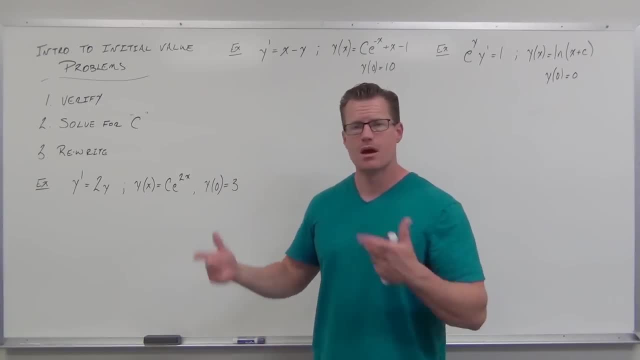 right there. So I'm going to show you how to do that on like six examples. The first thing I'm going to do completely for you, the next three I would like to do for you to do on your own Practice, this stuff. They're a little bit more advanced, but 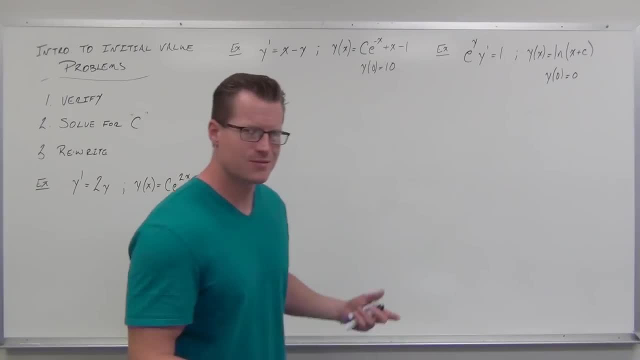 you should have the hang of it by the time you finish these three. So step number one: let's verify it. Let's make sure that in this first order differential equation, this is actually a solution. What that does remember the last video. 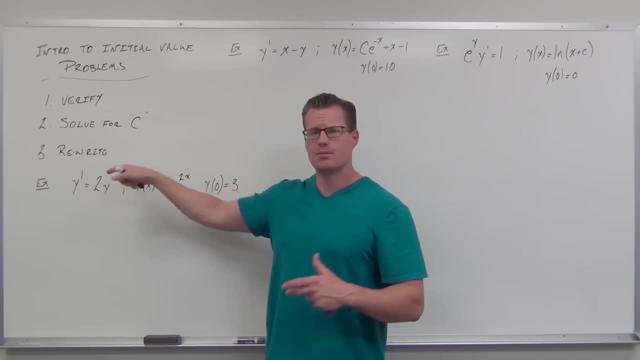 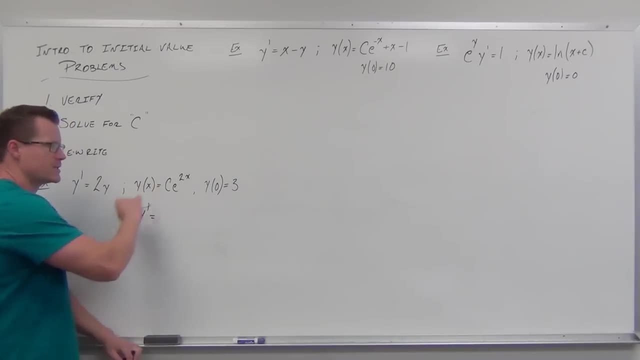 we have to take the derivative- thankfully only one of them- and plug it in to see what happens. So if we take the first derivative, C is a constant. It doesn't have any X's in it, So it's just a number. That means that we don't have a product. 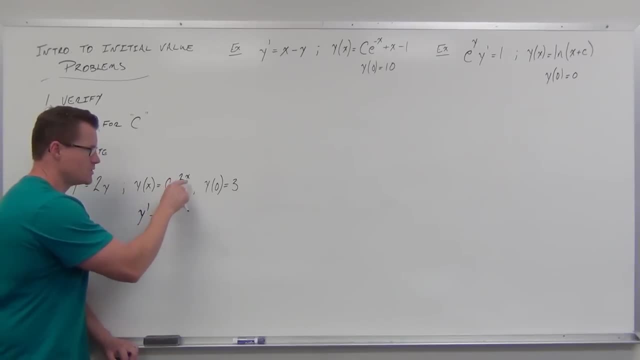 rule here. All we have to do is keep the C do this chain rule. Derivative of 2x is 2.. Just multiply in the front. you're good to go. Now let's plug this in. We're going to take our first derivative. 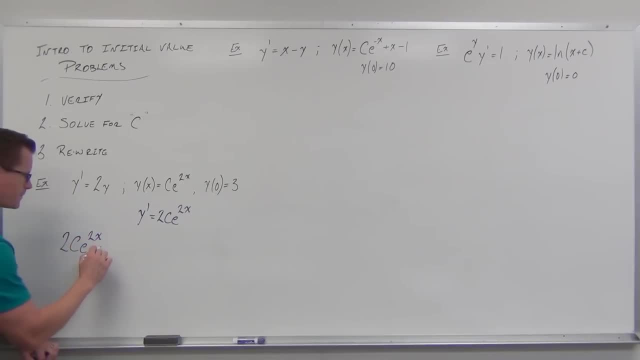 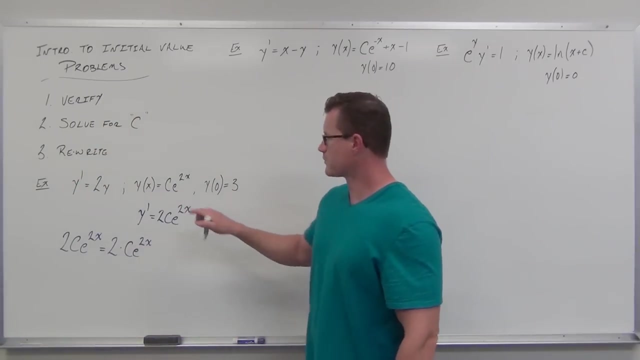 We'll see if that's equal to 2 times our original function. Yeah, that's like immediately apparent that those are. those are equal, So we know for sure that that's an actual solution. We've just verified that that's a solution to that. 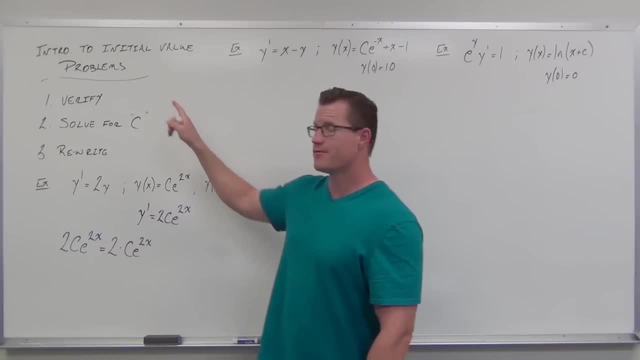 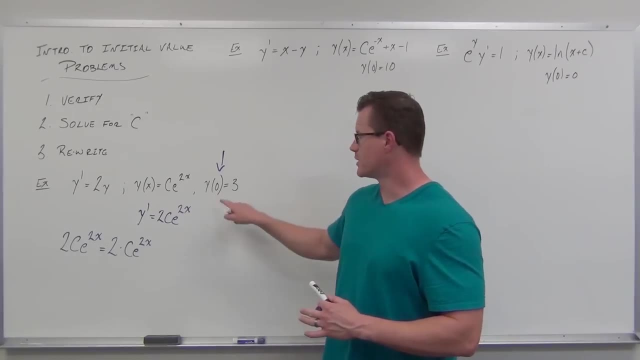 differential equation, Step number two. once you have verified that, solve for C. This is how you solve for C. So we're going to take and plug in: Y of 0 equals 3.. Now what that means is that Y of 0, what's Y of 0?? Well, Y of the independent variable X equals this. 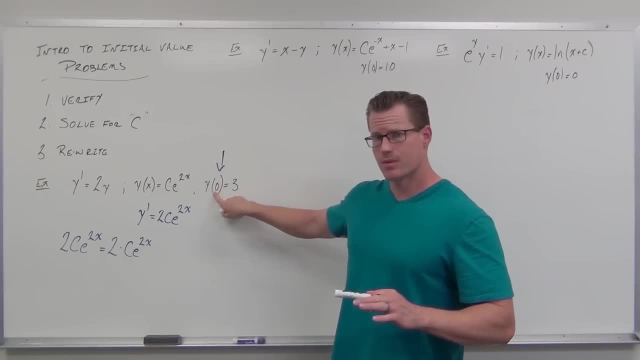 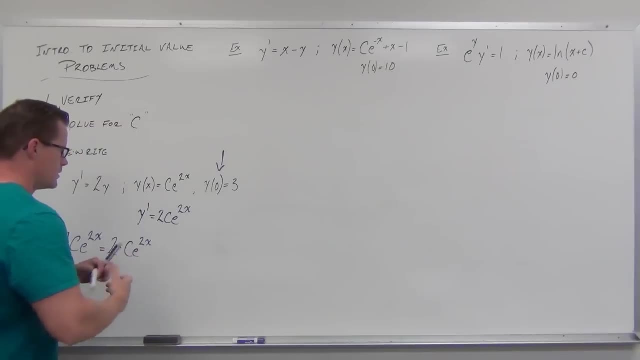 number. So replace X with that number, replace Y with that number and see what happens. So I'm going to start you off here. Let's replace X. even shows us what this is. It says: if you put in 0 for X, well it's. 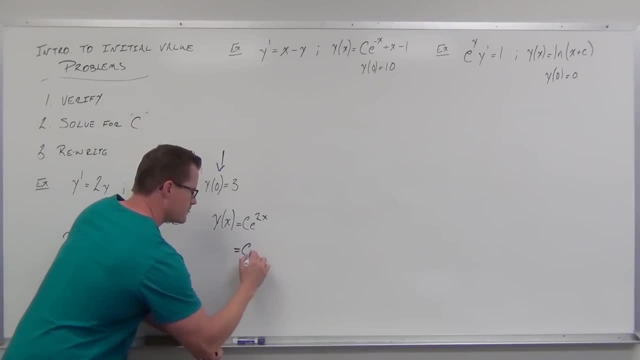 going to be equal to 3.. So if you put in 0 for X, it's going to be equal to 3.. That's what that means: Replace the X with this number, replace the Y with this number. That's exactly what that means to do, And that's that allows us solve for C. So if we 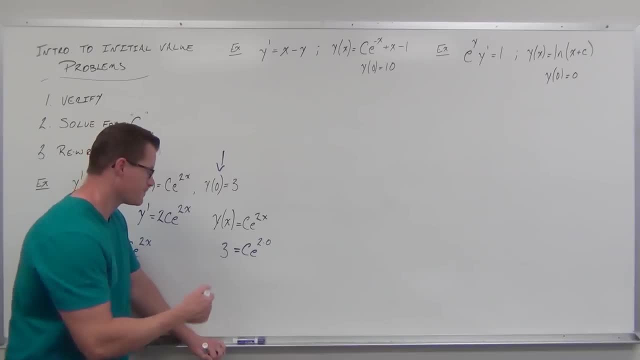 replace all the X's with 0 and all the Y's with 3, C equals one-third. Now, man, we're almost done. All we're going to do is replace the C in our original equation, our solution equation that we verify, with whatever C you found. So we're going to have: 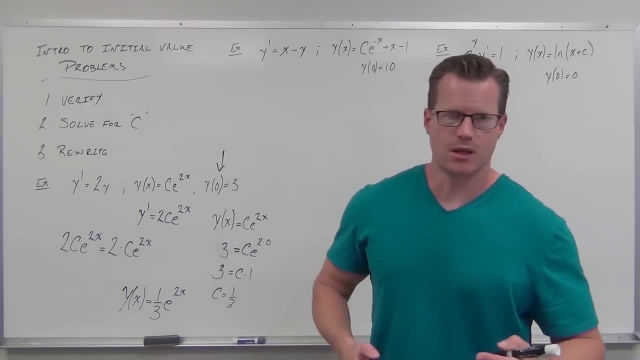 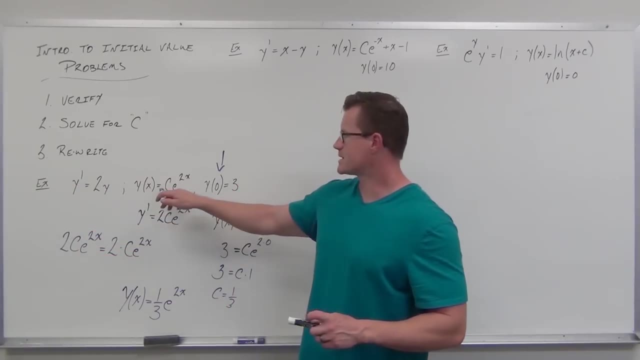 Y equals one-third e to the 2x. Let's walk through some terminology just to make sure you know what's going on. okay, That's a differential equation, It's a first order differential equation. This is a solution because we verified it. We know that that's a solution. It's a general solution because 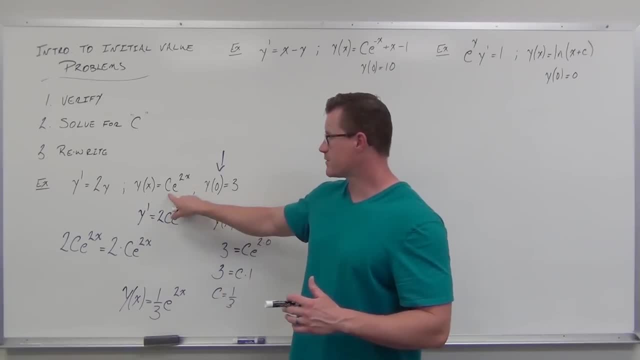 it's got that arbitrary constant in there. So this is a family of curves. Every single value of C is going to satisfy that. It's crazy. What we're looking for is now that we know that this is a solution. well, what's the solution? What's that curve that goes? 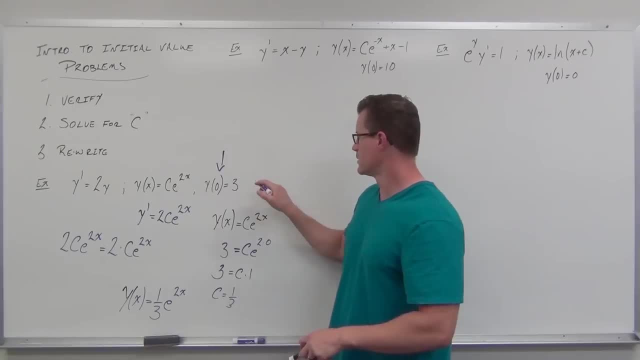 through that point. Another point: Yeah, that's the point 0, 3.. So notice, if you have a family of curves, they look like this because they're exponentials. If you have a family of curves, or like this: 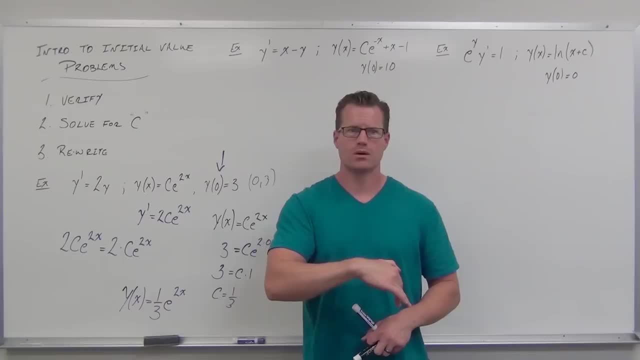 if that C is negative, all those exponentials. well then, if you have all that, what's the one of them that goes through 3, 0? And that's what we're asking. Oh, this one That goes through that point: 3, 0.. That's what we're doing. 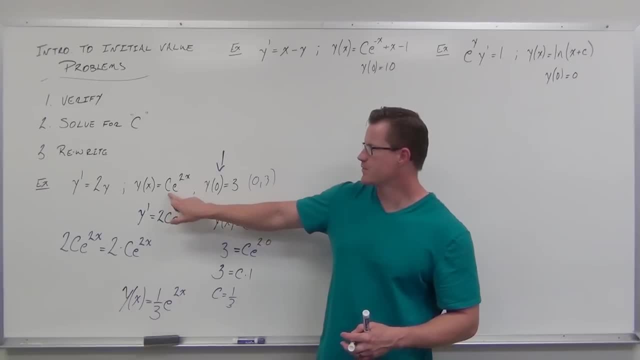 Let's think about the wear and tear of two lines between one equation to another and this product to this equation. Let's do that right, Let's do that. So this is equal to 0, 0, 2, 0, 0, 2, 1.. That's theoretical equation. 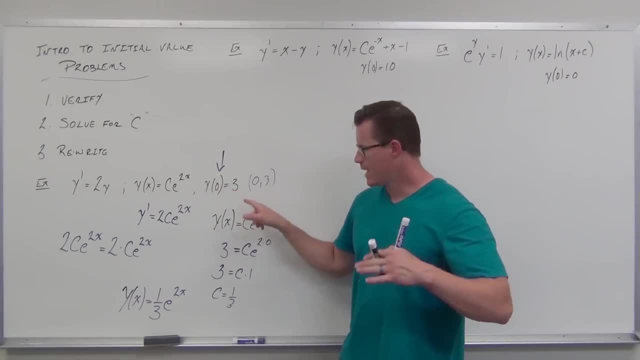 This is programming And that's why we're looking for something that's just going through things. by everything that's going, It's because this flag is too important to be considered real during Ancient blessing. OK, If you have a question, you're going to ask. 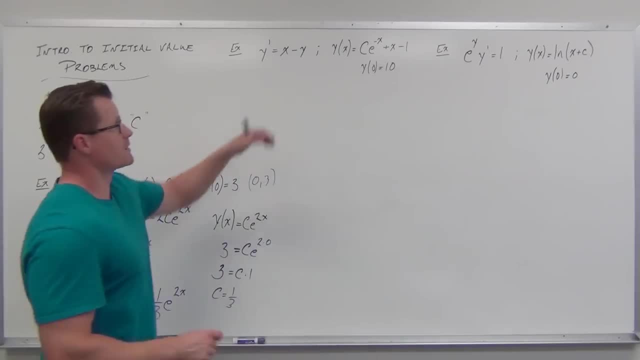 FR. You guys have gotten things out of this one right. How do we know for sure that we know exactly where we want the question to go? Is it now a problem with the equation? We need now give it a shot, Seriously. 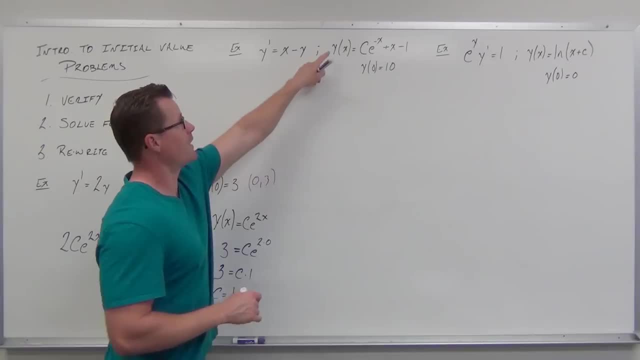 Don't let that worry you. All you're going to do is the same exact thing: Find the first derivative, plug it in, plug in the original to make sure that it actually works. So verify it and then use your initial condition to solve for C. So we're finding the first derivative to use here. 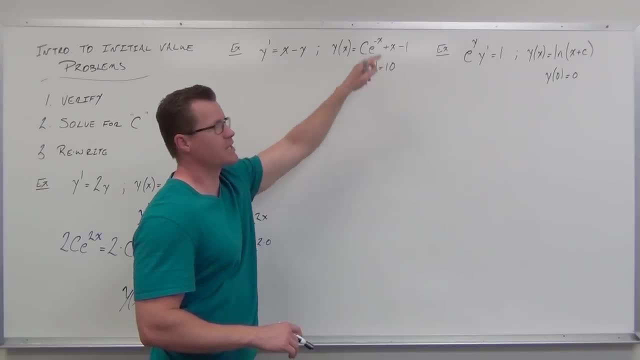 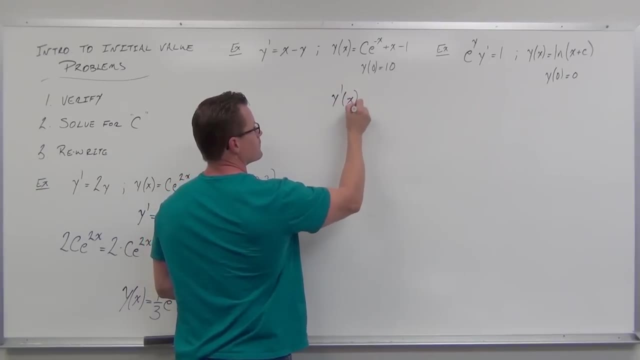 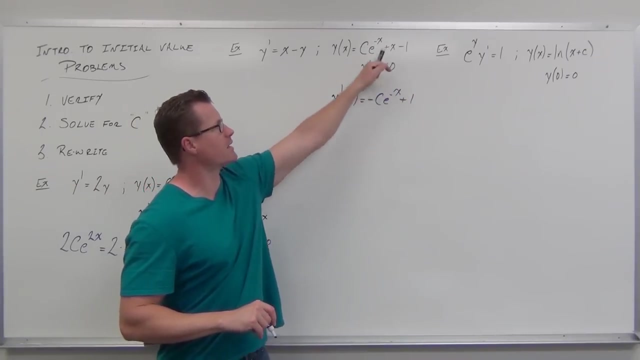 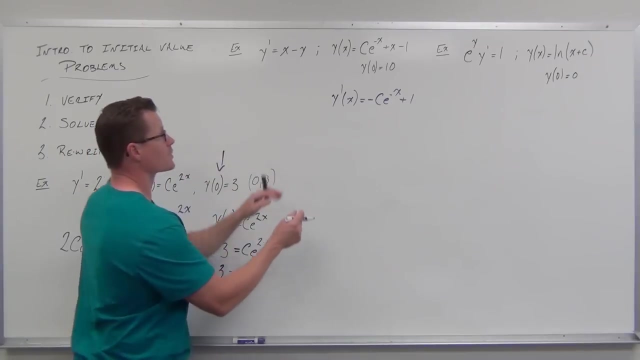 just to verify it. This is going to be reused in our equation that we're checking right now. So the first derivative chain rule gives us negative C e to the negative x plus one. This goes to zero. We're going to check this with our original in our differential equation to verify that this works. So on the 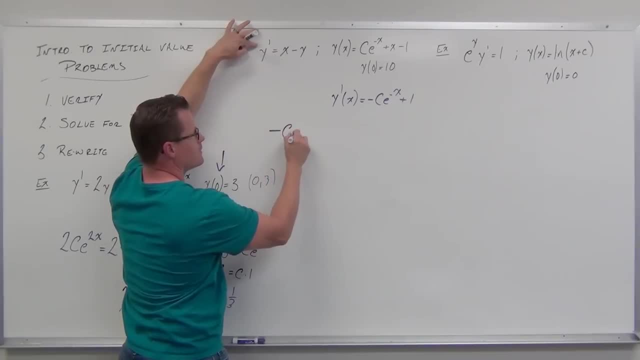 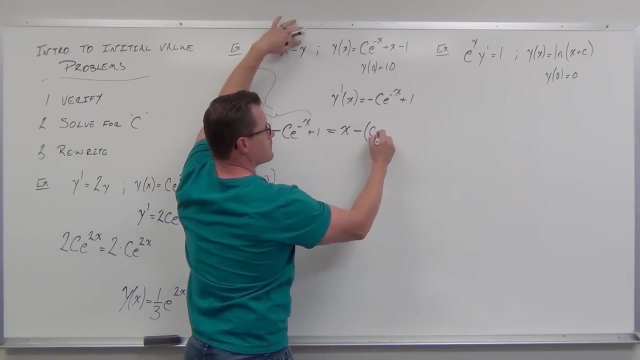 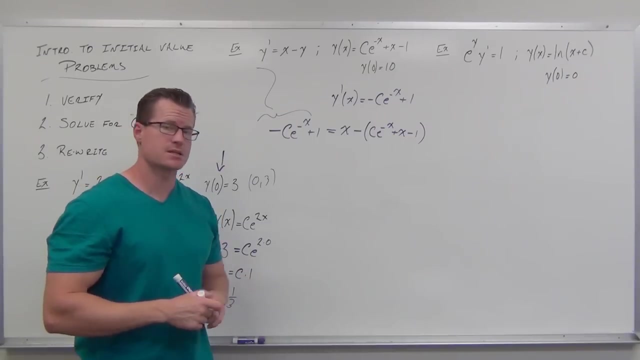 left-hand side. we're taking our first derivative. What we just found equals x, Minus our original equation that we just took the derivative of, And we're going to simplify this to see if what they've given us is actually a solution. It doesn't make sense to 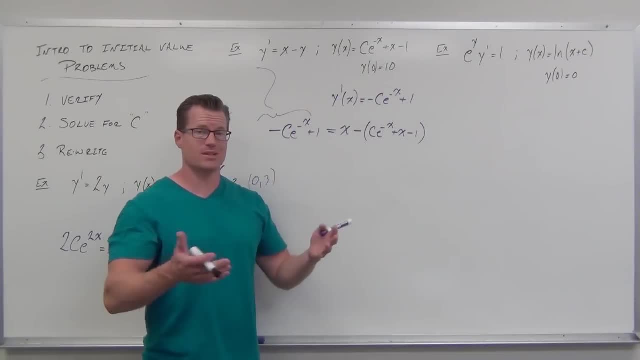 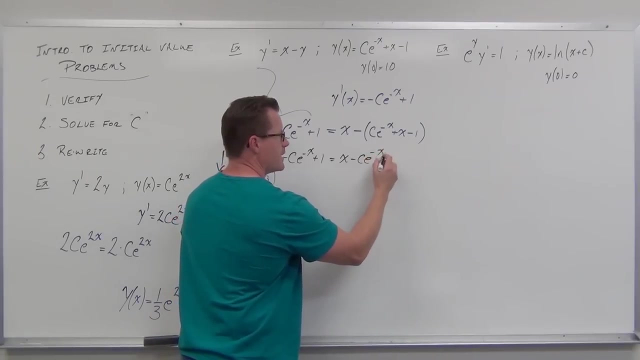 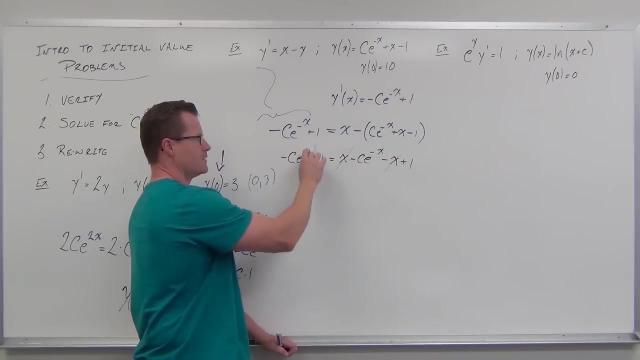 start plugging in initial values if that's not a solution, Because then you'd say: oh, this is not a particular solution to that differential equation. That is a waste of time. So we're going to make sure this works. If we distribute that minus, we get: x's are gone, B's are gone. One equals one. We nailed it. 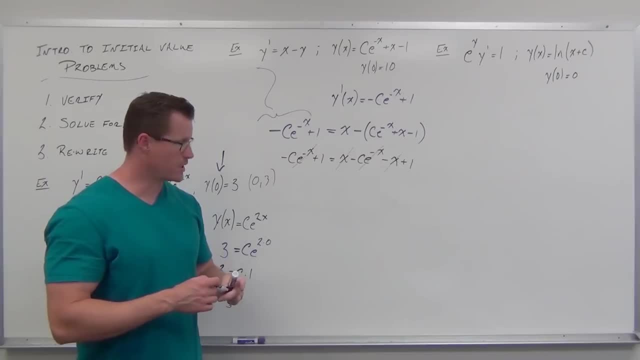 That is a solution to that first order differential equation. Now what we have to do is just solve for C, So we're done with the differential equation part. We're not even looking at that anymore. We've determined that this is in fact a general solution to it. It's got an. 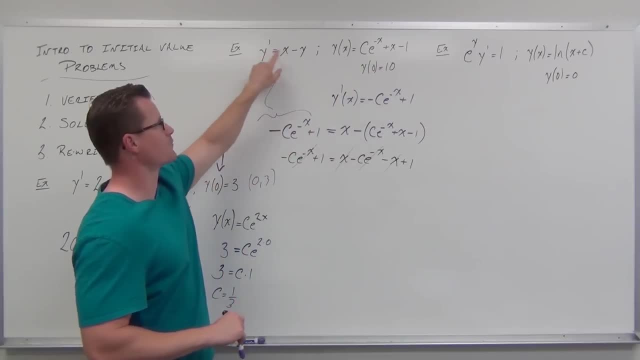 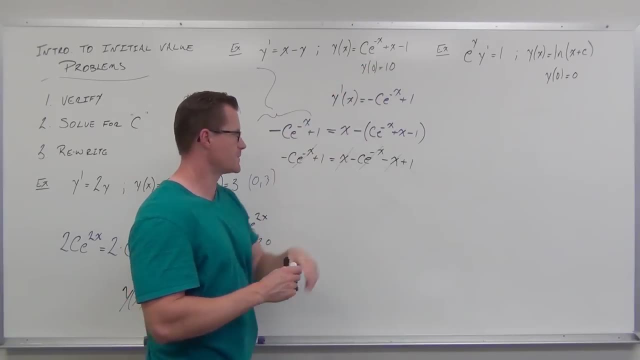 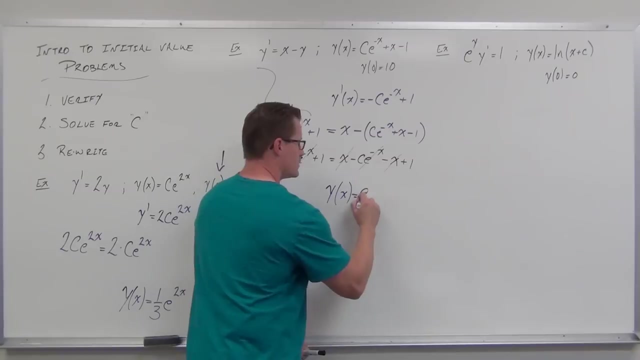 arbitrary constant. We only need one arbitrary constant. with that, It's a first order, one arbitrary constant. All we have to do now is, now that we've verified it, plug this initial condition in and solve for C. So I'm going to rewrite what we're doing here, Our solution, our general solution. 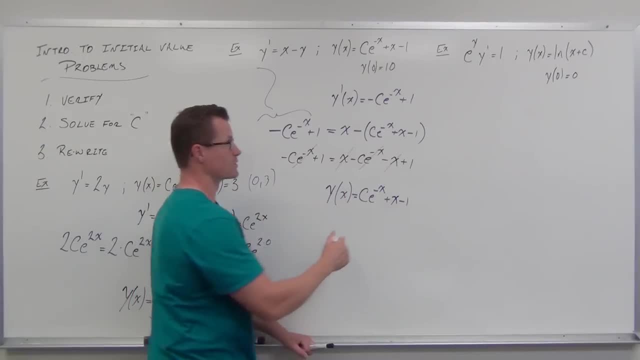 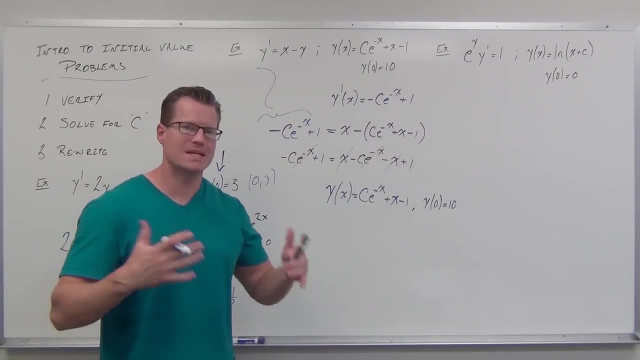 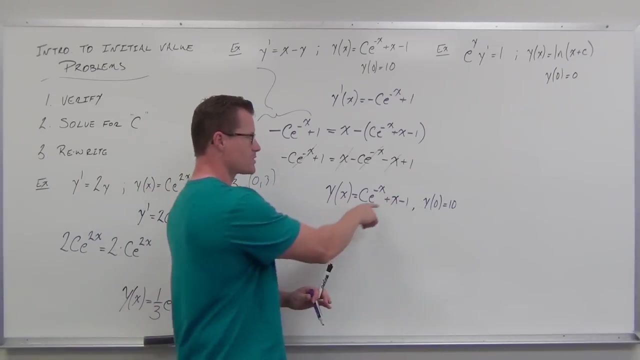 is this Our initial condition? we know that's a general solution. Our solution is the initial condition or the point that we need our solution to go through. We have to have it satisfied by that. It's going to give us a specific C. All these are: 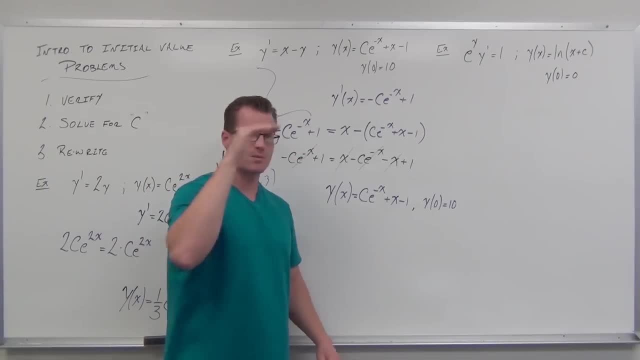 different curves. They look like a whole stream of curves in a graph, but only one of those is going to go through that point. The C value is what gives us that one curve that goes to that one point. Hopefully you see it. x is going to become 0.. y is going to become 0.. All of my inner. 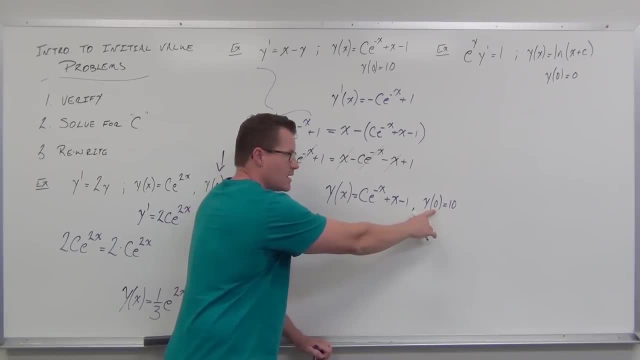 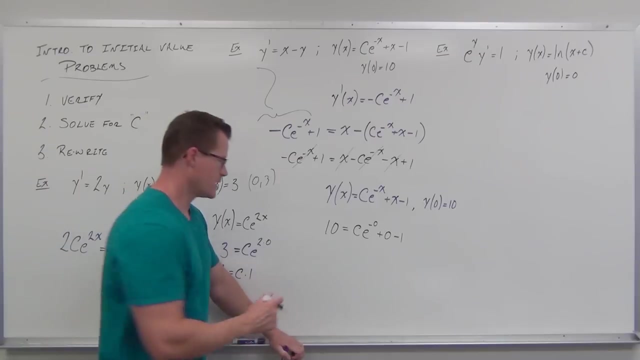 curves are going to muster up in the graphм. Now our solution is this: We've gotg the initial Cóndor and now we're having the initial condition point. we need our solution to go through to 10, and we're going to solve for c. So y is 10 when x is 0. Usually these work out pretty. 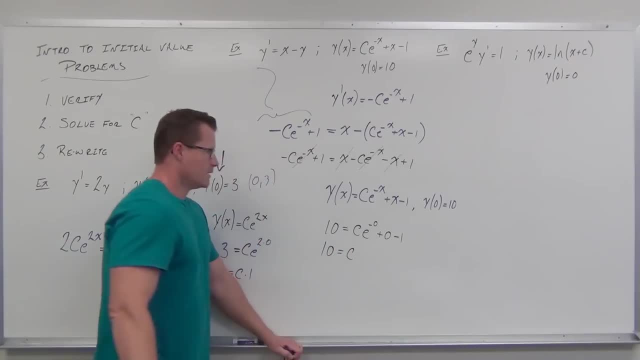 nice e to the negative 0, who cares? e to the 0, that's 1.. c times 1 is c plus 0 minus 1.. If we add that, 1 over c equals 11.. Let's just replace that, and then we're done So. 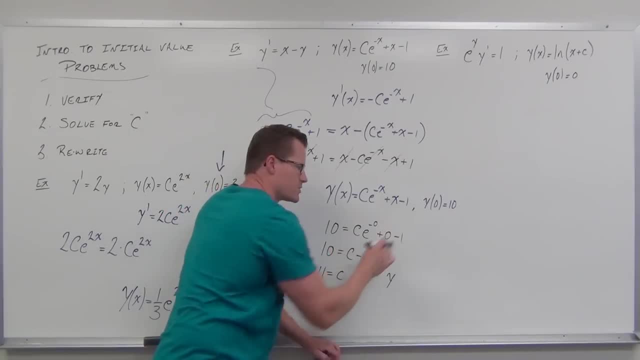 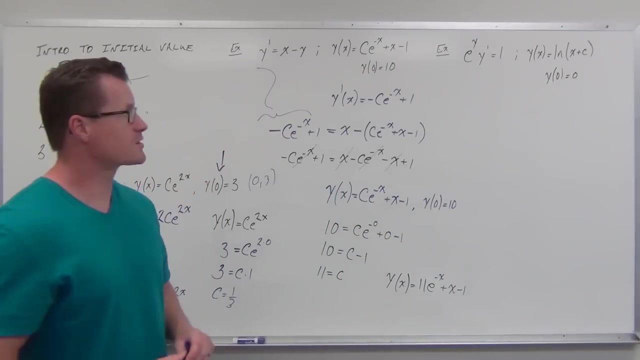 our particular solution, the solution that satisfies our initial condition from our family of curves here for our general solution to our differential equation is: y of x needs to be 11, e to the negative, x plus 0.. x minus 1.. That's the idea. I hope that's making sense. All right, let's try one more. 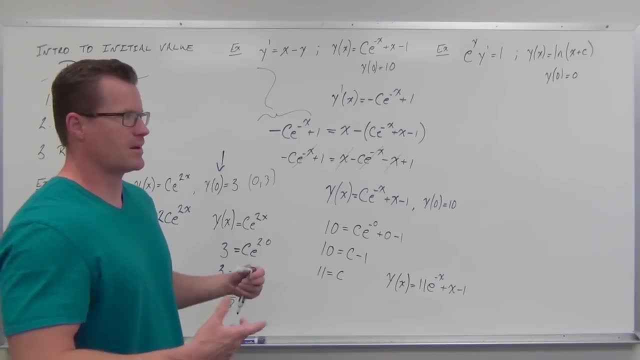 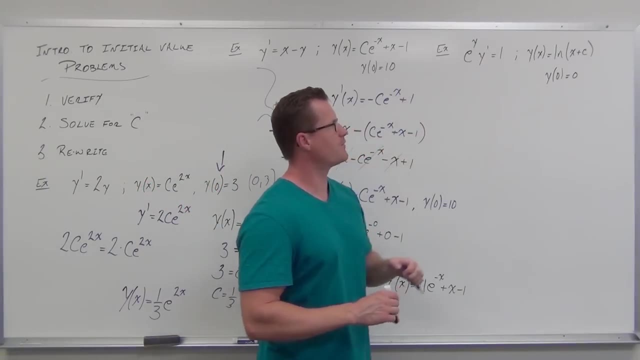 together before I give you like three more to do on your own, and then I'll of course go through them with you. So we do the same exact process: Let's find the first derivative, Let's plug these both in to verify, and then let's use our initial condition to solve for. 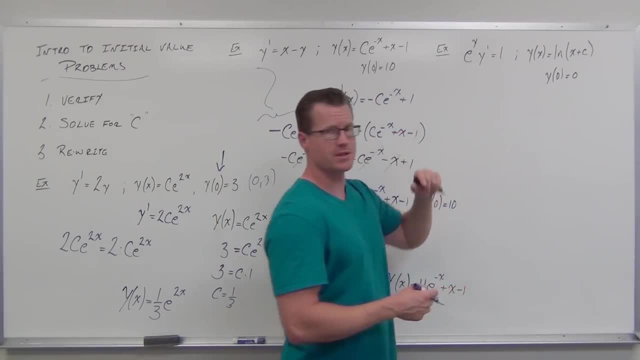 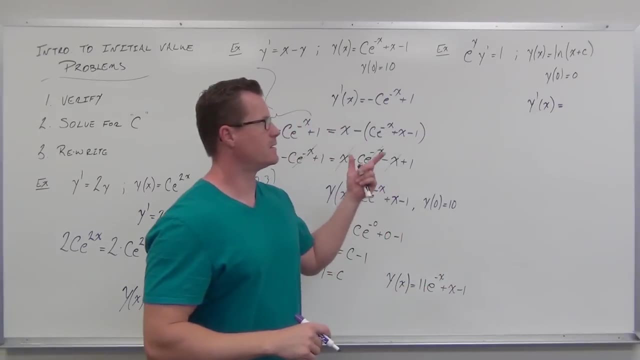 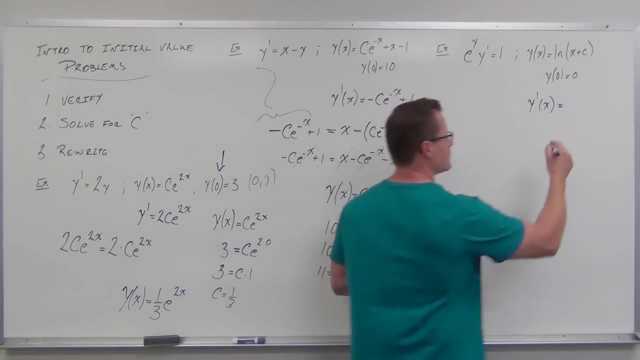 c. So first comes the verification. We need to take the first derivative to satisfy our differential equation. The derivative of ln of x is 0.. x plus c is 1 over x plus c times the derivative of x plus c. That's a chain rule, Since the 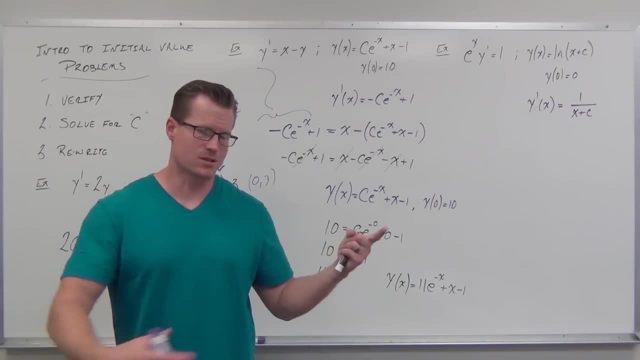 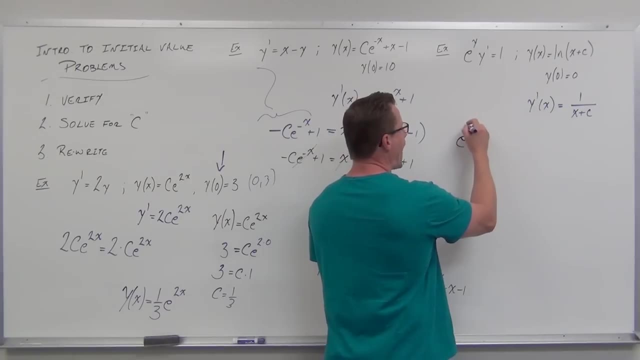 derivative of x plus a. constant is just 1, remember, constants go to 0, we just get 1 over x plus c. Let's plug that stuff in. So we're going to have e to the ln x plus c, That's e to the y. y equals ln x plus c. 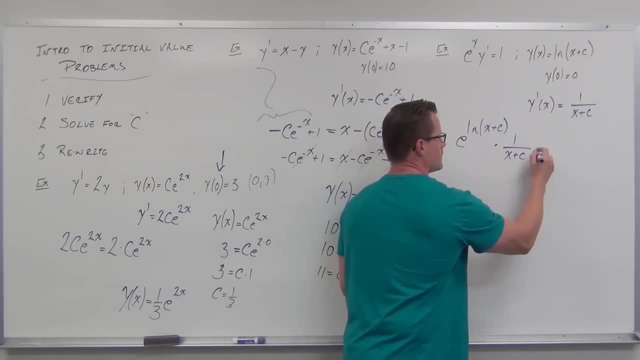 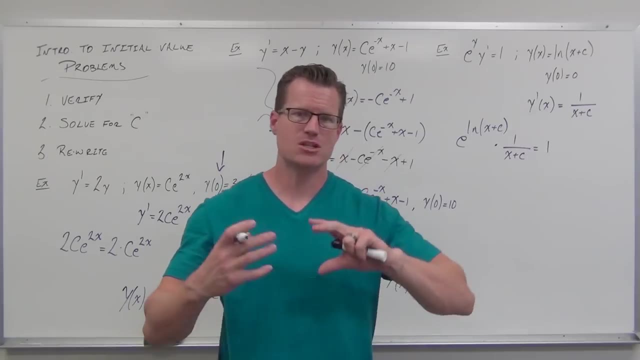 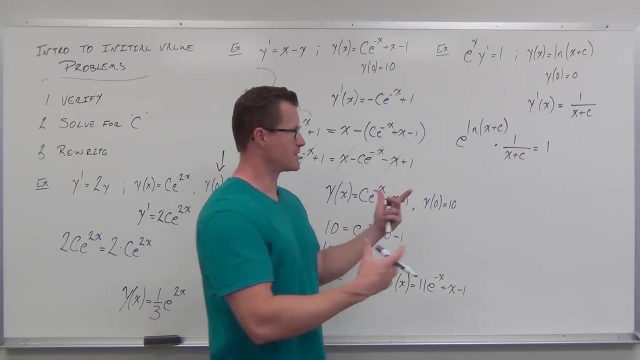 x plus c times the first derivative of y. We just found that and that's going to equal 1.. Well, if you remember identities e to ln, that sort of idea- those are inverse functions, Those are an exponential and logarithm are always inverses if they have the same base. 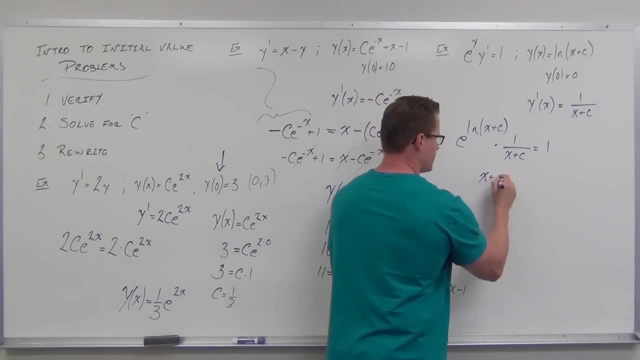 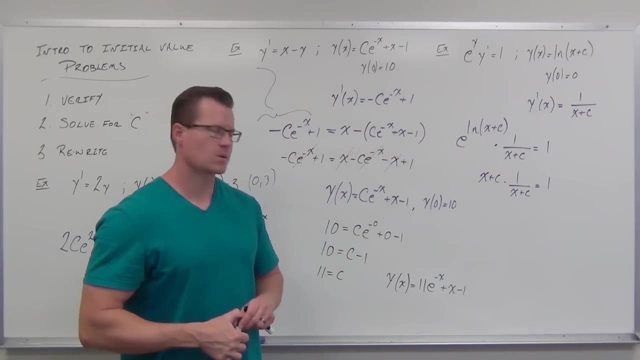 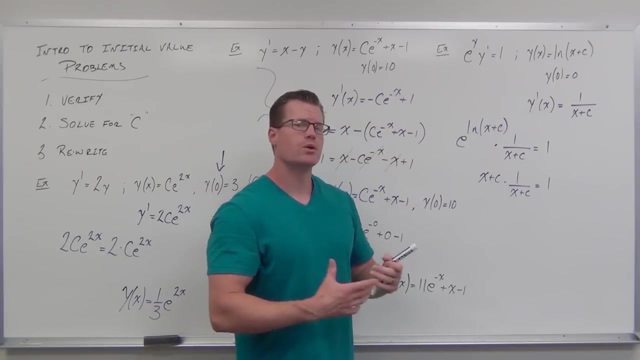 That's all gone. We're going to get x plus c, And x plus c times 1 over x plus c. that's certainly going to equal 1.. So we know that that's a solution to that differential equation. Now we're going to use our initial condition, so I'm going to rewrite it. 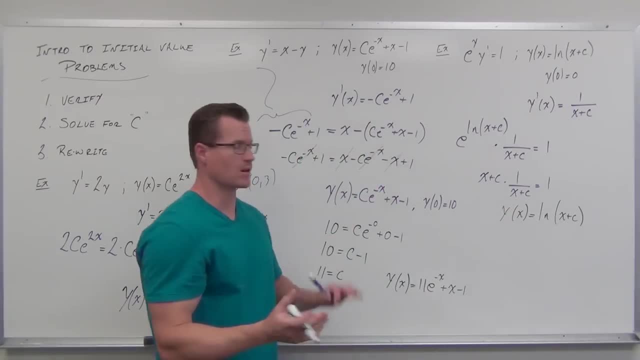 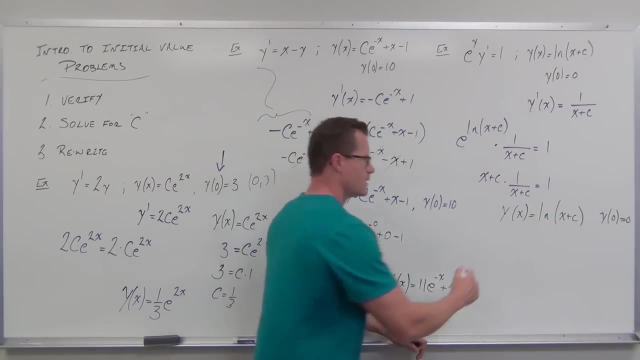 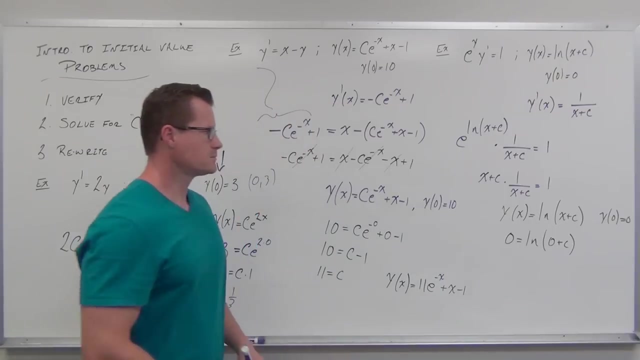 So we have our general solution. It's got a c in there. Plug in your initial condition When x is 0, y is also 0. So 0 has to equal ln of 0 plus c. 0 has to equal ln of 0 plus c. 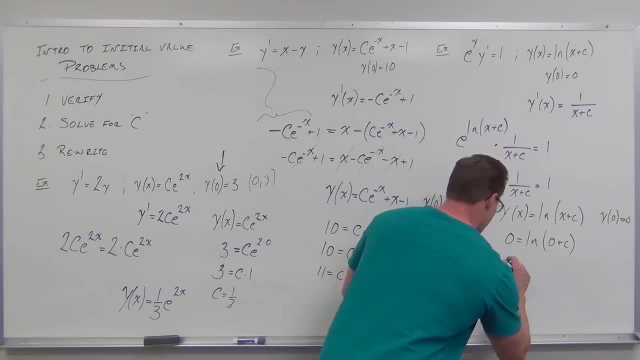 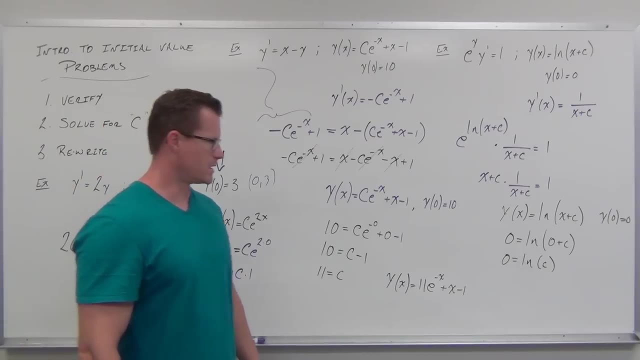 We have 0 for y, we get 0 for x. That looks weird. So 0 equals ln c. Let's do an exponential on both sides, Or just think about it. What value of c does there need to be there in order for ln to equal 0?? 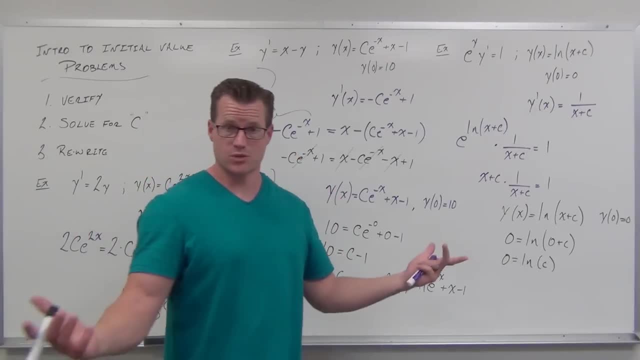 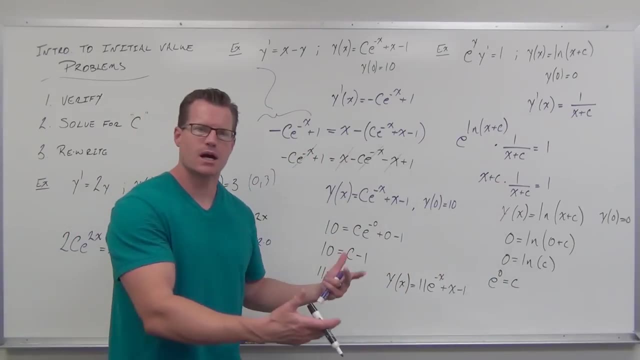 ln of what equals 0? We go 1.. Yeah, c is going to be 1.. So if you need the exponential e to the 0 equals c. Do an e on both sides, or think about the inverse of ln. 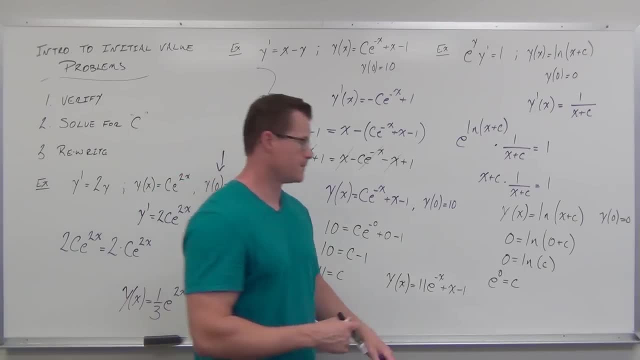 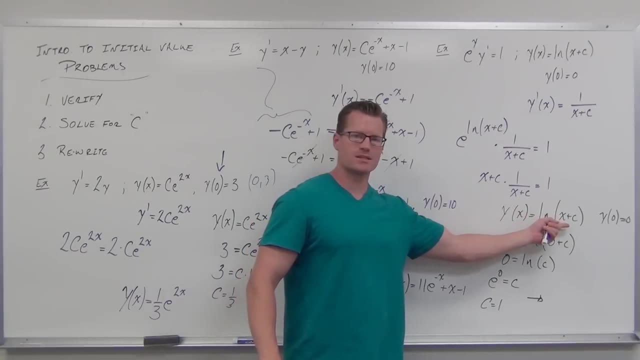 It's an exponential. e to the 0 equals c. c has to be 1.. Which means now we go back and we just replace our arbitrary constant with something that's not arbitrary anymore, something that's particular, something that says: hey, you're going through that point. 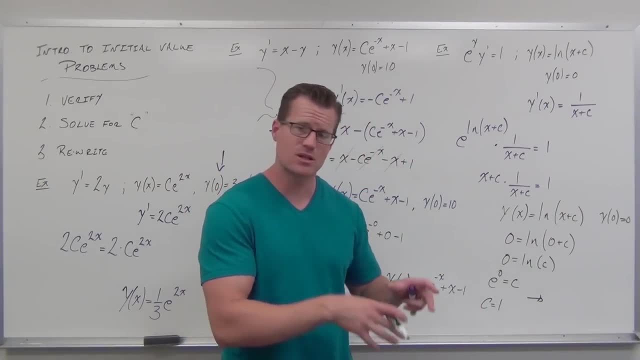 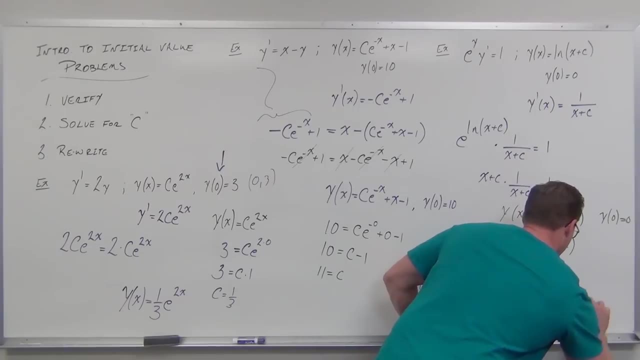 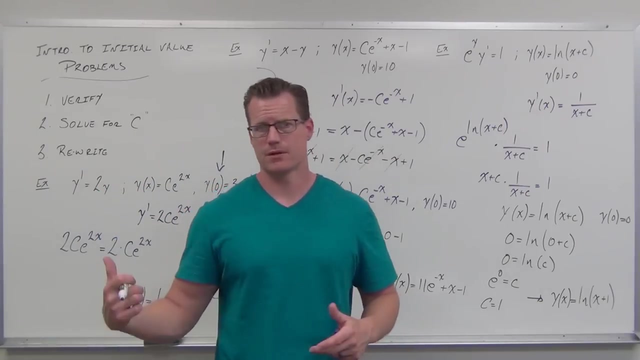 You don't need an arbitrary constant. You have a specific constant that's going to let you go through that specific point, That initial condition, And that constant is 1.. That's the way that we do it: Verify, solve for c, then just rewrite it. 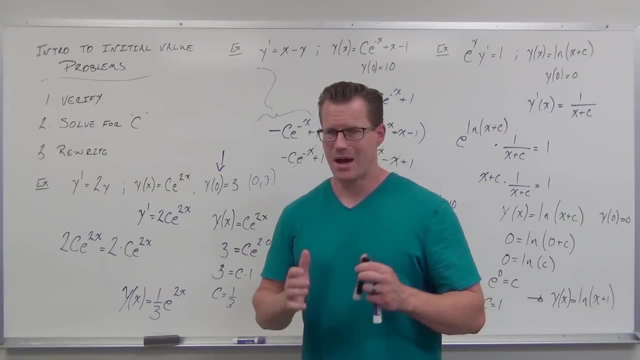 I'm going to erase the board. I'm going to put three more on the board for you. I would really encourage you to try them. See if you can verify, solve for c, rewrite. It's not that hard, but the process is important because we're always doing these two things. 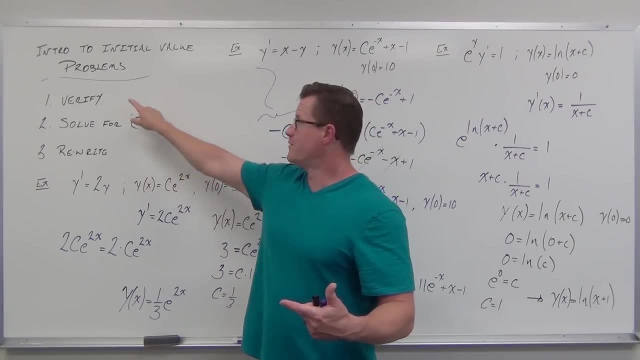 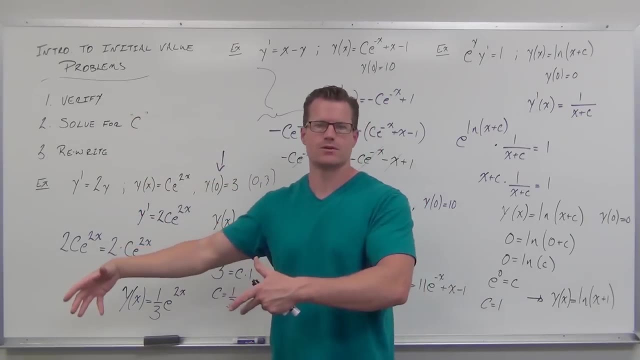 when dealing with initial value problems. Later on, the verify part: well, you're not going to verify anymore in a little while. You're going to be actually solving this, You go. oh, I solved it. Now solve for c. 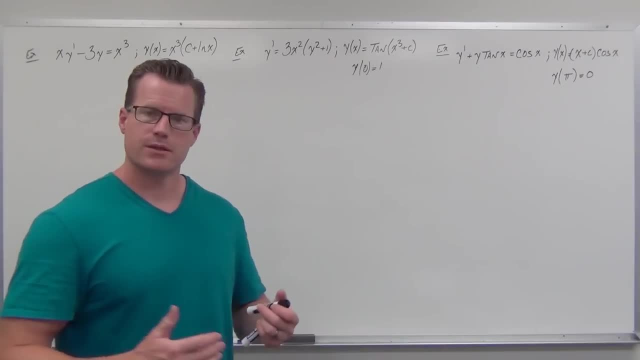 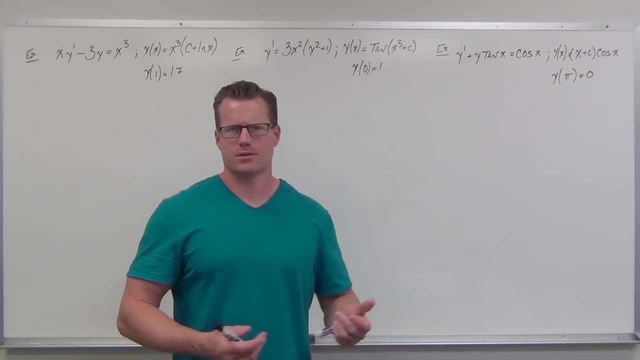 Now rewrite it. That's the way it works. So now that you have the hang of it, try these three problems. Yeah, they're a little bit more intimidating. There's more stuff going on, but don't worry about it. 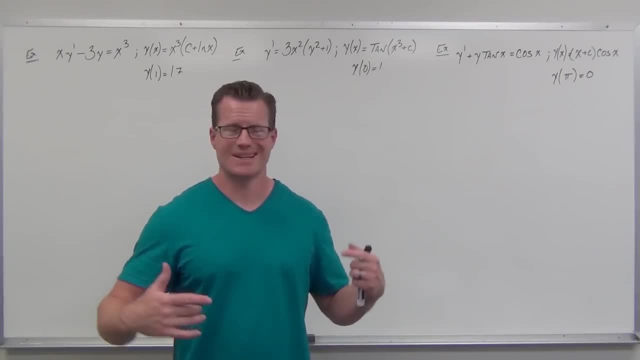 See if you can verify. first Take the appropriate derivative, plug it in, see that it works and then use the initial value problem. Some of you are probably thinking- but I trust you, I'm kind of out of my mind. I'm kind of out of my mind. 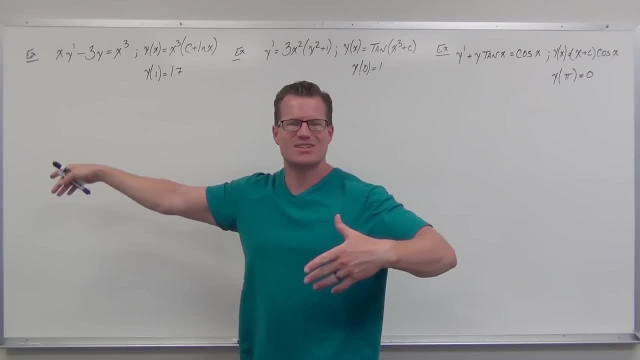 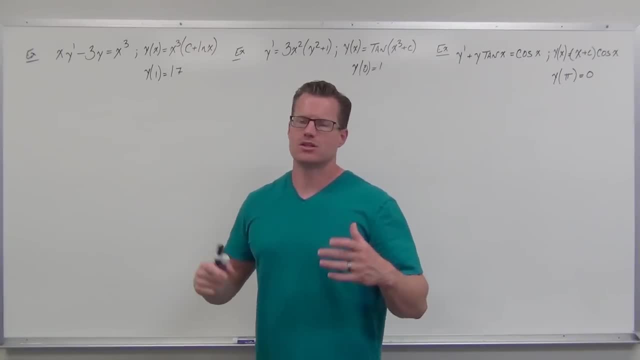 You can do that. You can do, you can find c. that way It's just good practice to verify it to make sure it actually works, because if it doesn't work, then that's irrelevant. So try it, Even though we're. it seems like we're kind of wasting time because you're like: well, 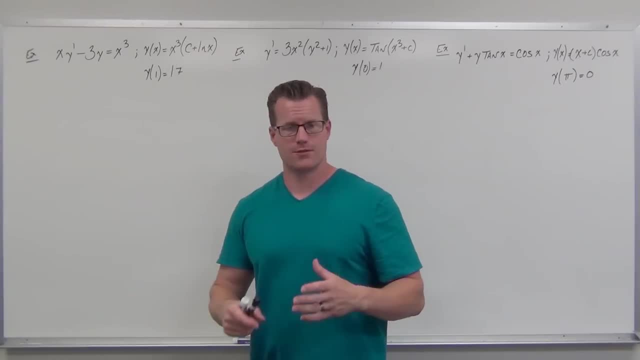 if they're telling me that's a solution, they're not. They're saying: verify that it is first. Trust me, that's a lot easier than finding that yourself. so finding that with the techniques later on takes a lot more time. So verifying is way quicker than actually finding the solution for yourself. 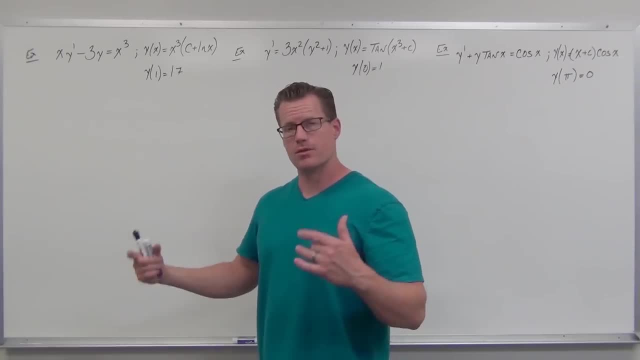 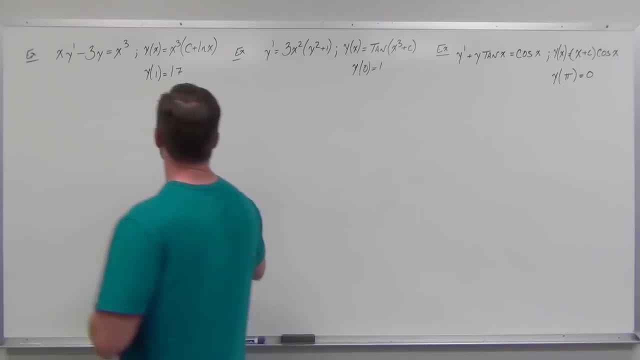 So take the time to do it, Verify it's actually a solution, then solve for c and then rewrite it. So I'm going to start right now. Hopefully you'll take the time to do that on your own. Step number one: we're going to find derivatives for everything. 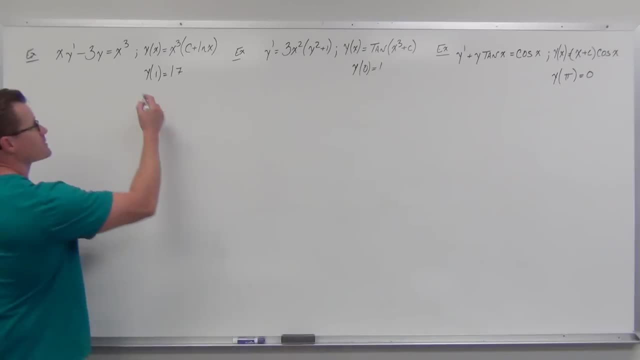 because they're all first order differential equations. That's kind of nice. Now, what we're noticing here, though, is there's got to be a solution, There's got to be a product rule when you're finding that first derivative. Here's a function of x. 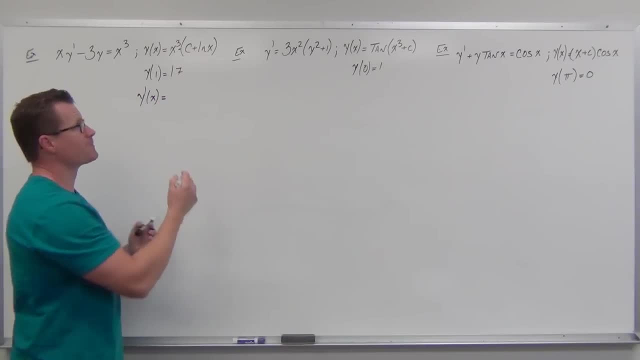 Here's a function that has x in it. We're going to have a product rule, So derivative of the first times, the second plus the first times, the derivative of the second, Now the derivative of the second, derivative of the constant that's zero, so that it's not one. 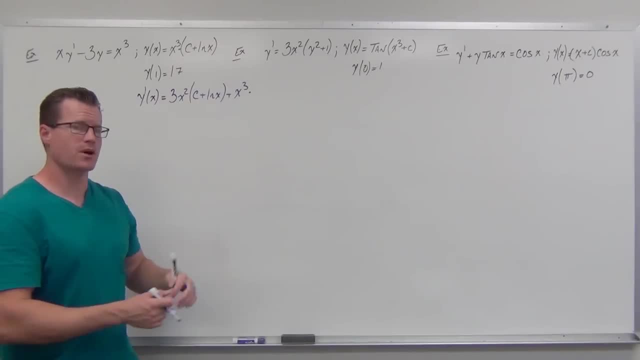 It's not that it's zero, It's gone. The derivative of ln x is 1 over x, So that's what we're going to be plugging in here. Let's go ahead and do that. So when we verify this, we're going to take our first derivative, put it here. 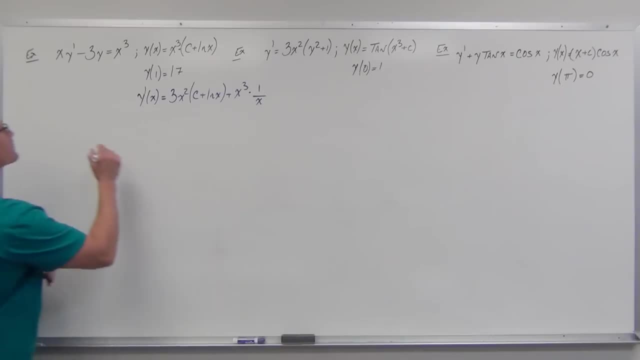 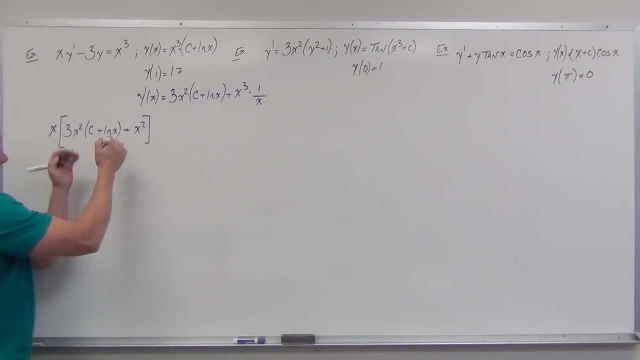 And notice how this is going to distribute to all of this. This is all the first derivative that needs to be in brackets. Let's distribute. Let's see what happens. If we distribute this, we're going to get 3x cubed times some nasty stuff that we don't really want to look at. 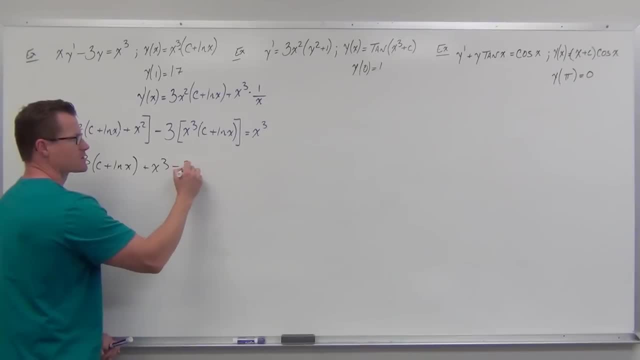 plus x cubed. But here when we distribute we get minus 3x cubed Nasty stuff that looks exactly like the other nasty stuff. I like that Equals x cubed And we can see just on some observation here that this and this are gone. 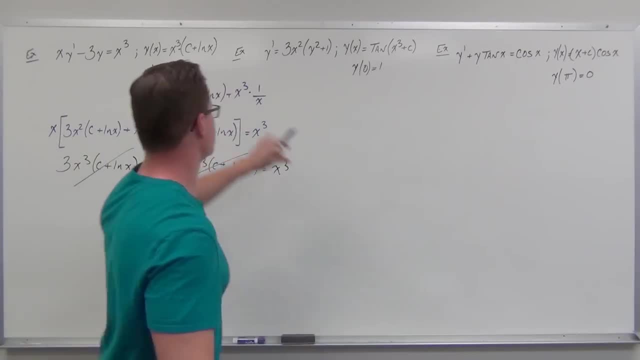 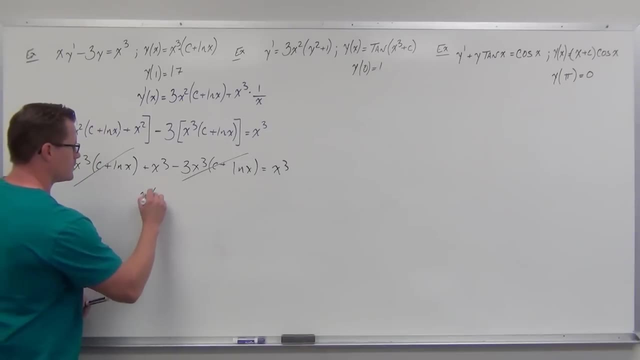 x cubed equals x cubed, And we win. So we know that this, right here, is a general solution to that differential equation. Now, now it's appropriate to find c. It might seem pedantic, It might seem like a waste of time. 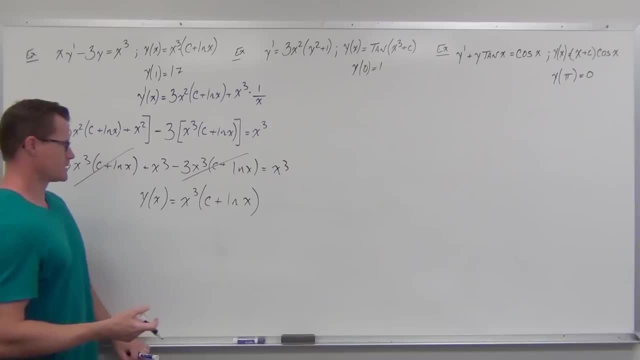 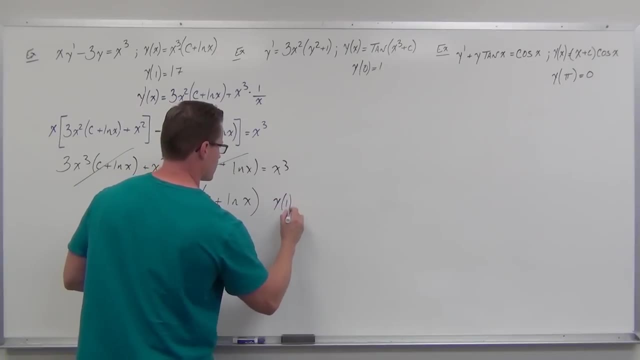 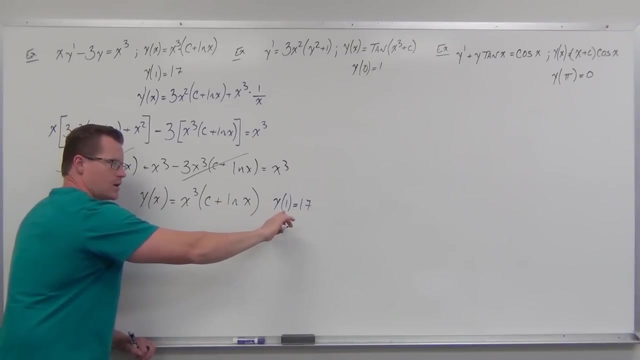 I know it would have When I first took it to think like, well, it's going to be a solution, But it's important to verify that. So when we plug in, we know that when x is 1, y is 17.. 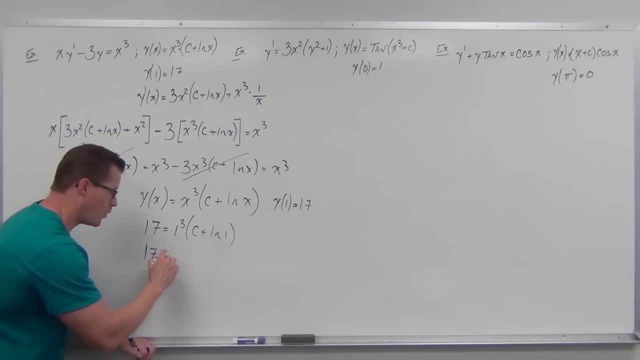 Well, so 17 equals 1.. 1 cubed is 1.. ln of 1 is 1.. 1 cubed is 1.. 1 cubed is 1.. 1 cubed is 1.. 1 is 0.. 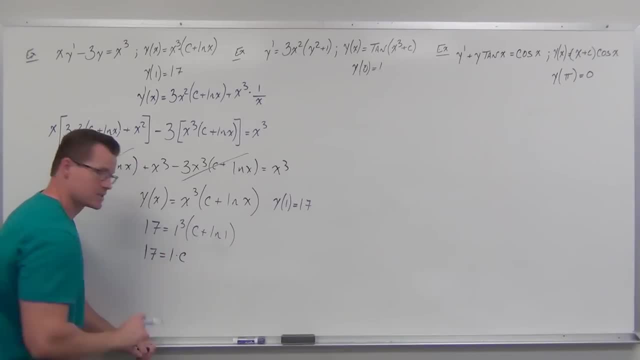 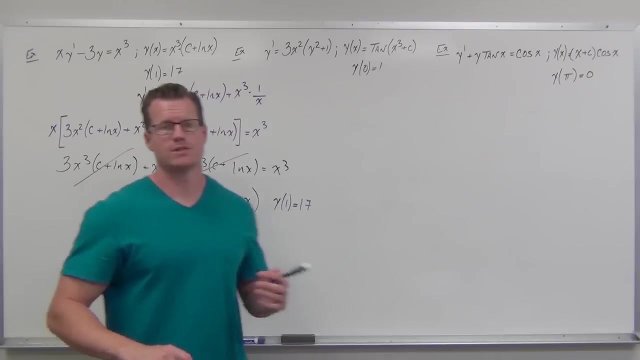 We just talked about it a little while ago. 0 plus c is c, So c equals 17.. That's it Now. all we got to do is replace that with 17. And we're done. We've taken a general solution with an initial condition. 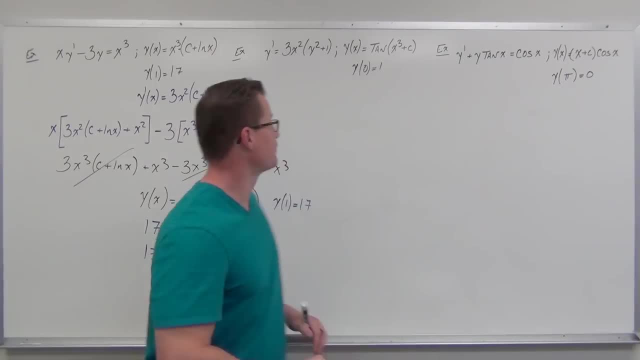 and found a particular solution to that differential equation. That's it, OK. next up, we're going to take the first derivative to make sure that we verify that this is actually a solution here. Wow, that's crazy. Do you remember the derivative of tangent? 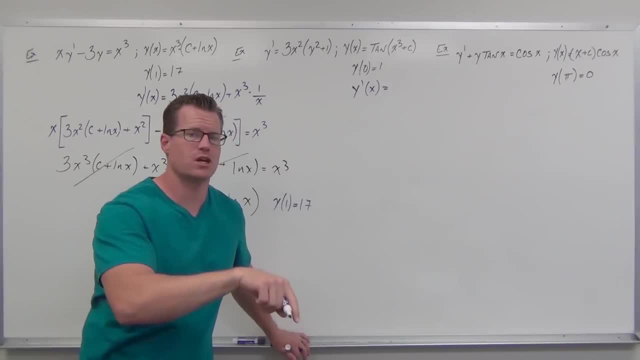 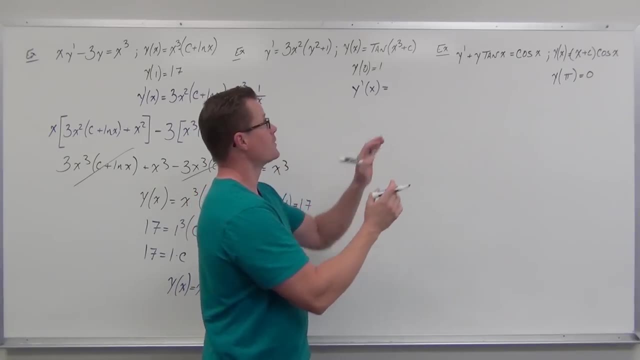 How did we do? Derivative of tangent is secant squared, But then we have a chain rule involved in that, So secant squared of the original stuff times the derivative of the inside stuff. The derivative of this is 3x squared plus 0.. 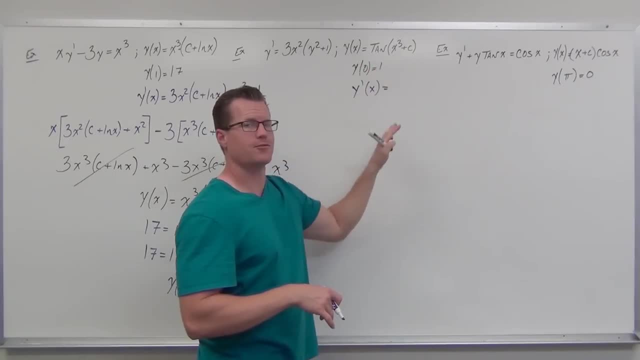 Derivative of constant 0.. So this is 3x squared And we're going to put that in front of secant squared of this stuff. So we would get secant squared. Leave the inside alone. Times the derivative of the inside. 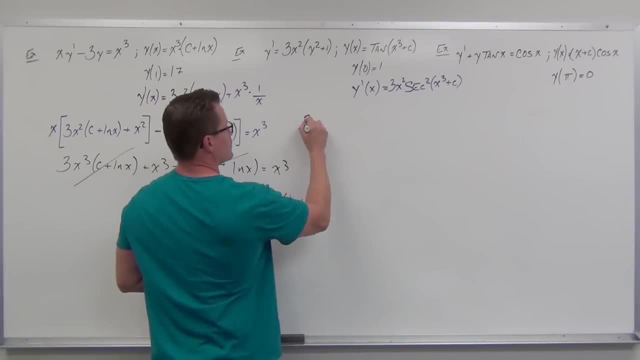 That's 3x squared. That's it Now. plug that in. 3x squared. secant squared x cubed plus c equals on the right-hand side. we have some more things going on here We're going to have. let's see. 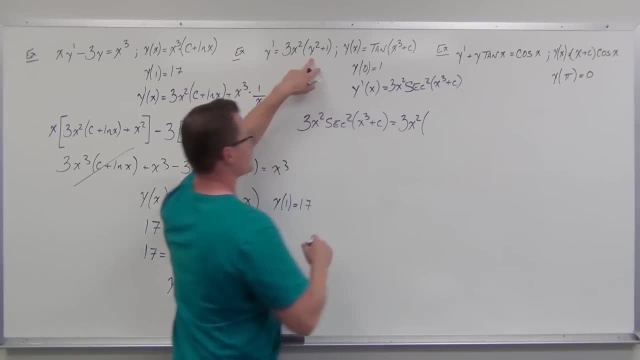 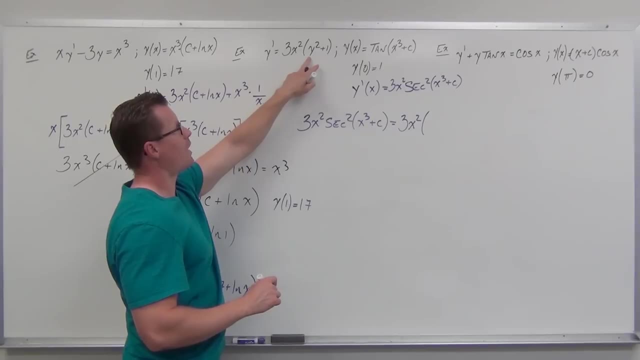 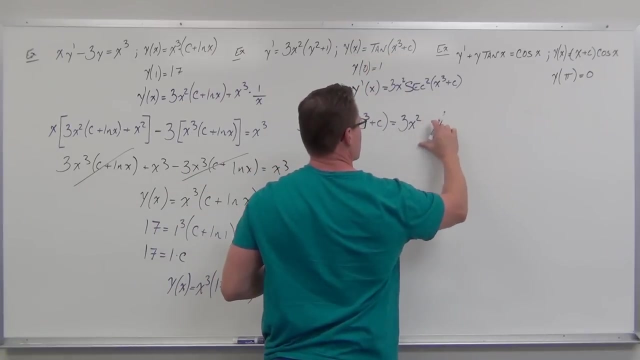 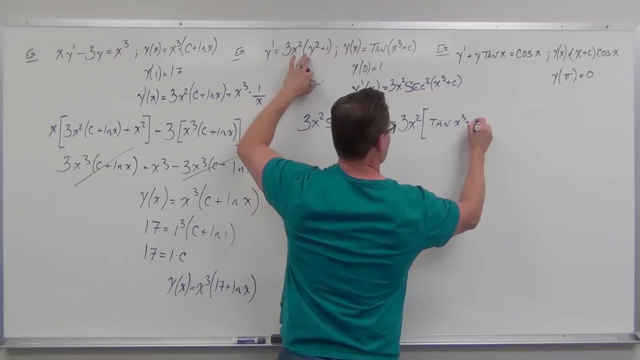 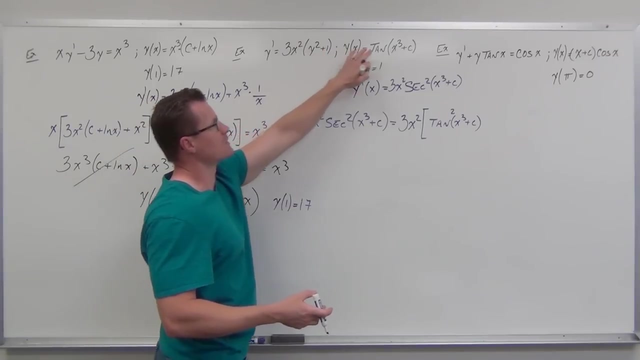 Three times 3x squared, Three x squared, So that's good. We have y squared, Y squared, So all of this squared, So tangent squared. Why? Because that's why you're saying y squared, That's y, So y squared. take this stuff and square it: Tangent squared of x cubed plus c plus 1.. 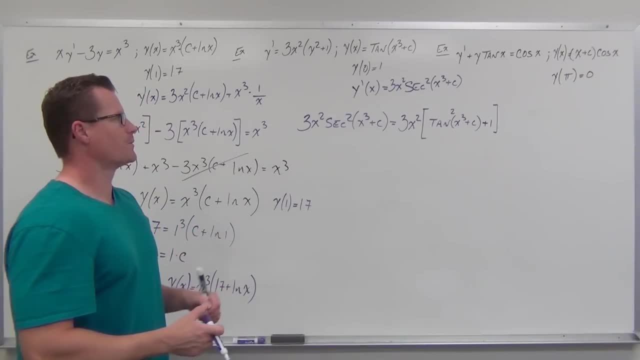 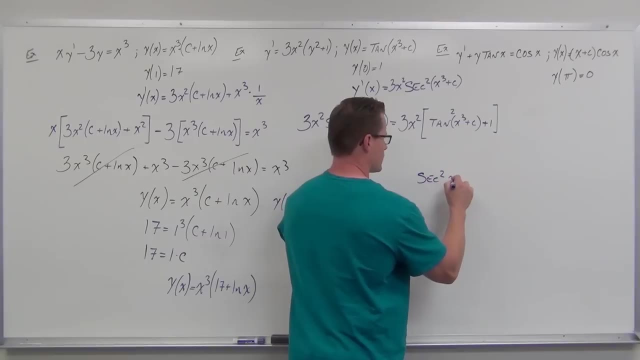 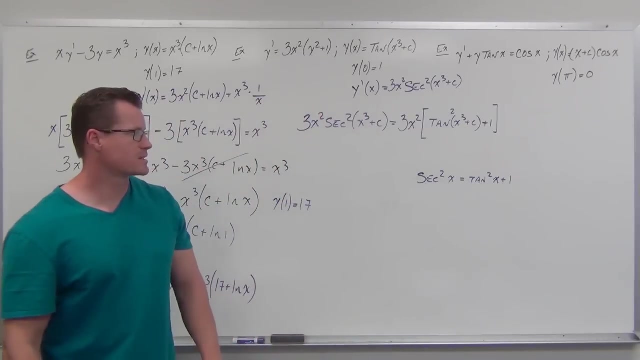 That doesn't look the same. Well, we have to remember some of our identities, So some trig identities are that. That works, So secant squared x equals tangent squared x plus 1.. What that means is that this right here is really secant squared x. 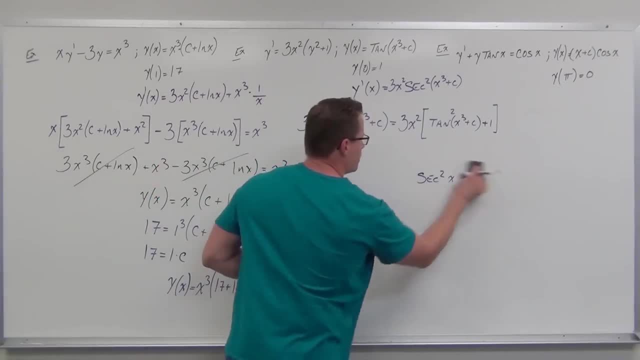 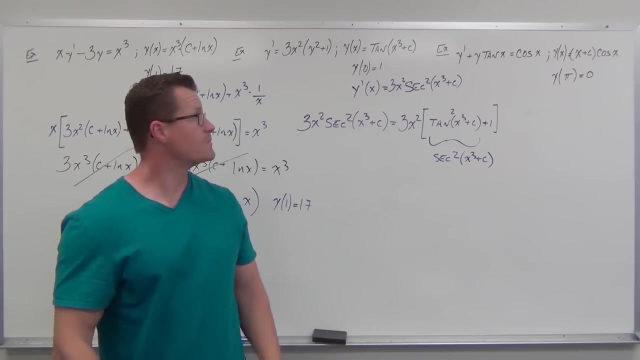 That plus 1 disappears because of our identity, Which means that these things are identically the same. This is secant squared x cubed plus c. This is secant squared x cubed plus c by that identity that I just showed you. 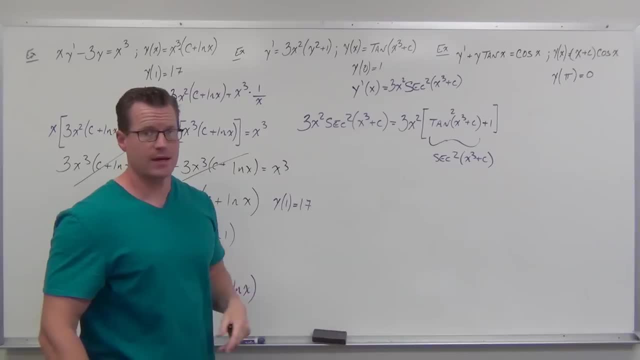 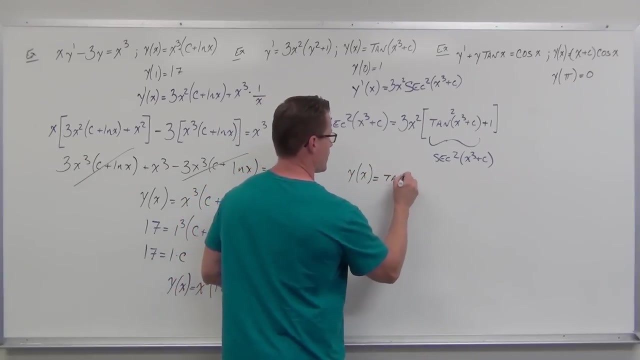 So that verifies that this is a solution to that first order differential equation. Now it's on us To find c and then rewrite our original solution as a particular solution. So let's do it. We got y of 0 is 1.. 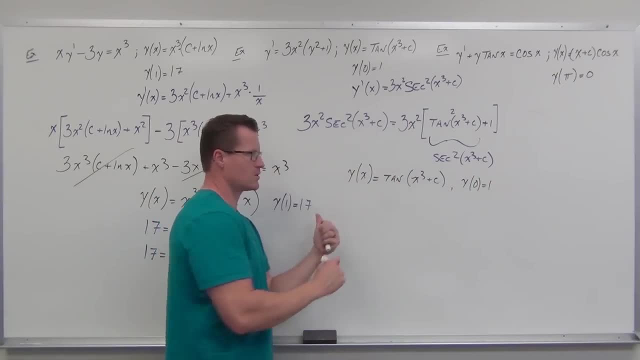 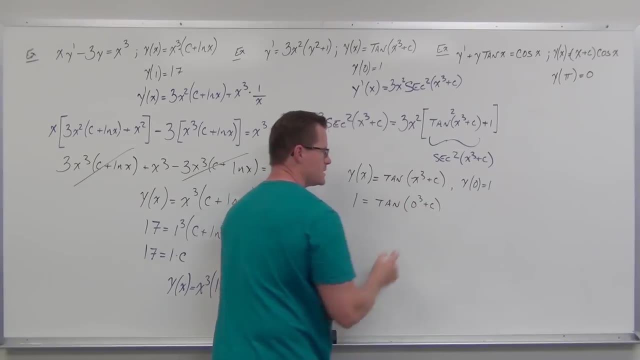 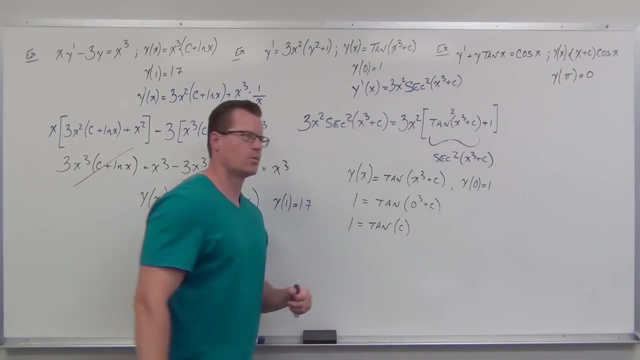 That means that every time x is 0, y is going to equal 1.. So 1 equals tangent of 0 cubed plus c. Okay, What value? What's it take? What's c got to be for tangent of that value to equal 1?? 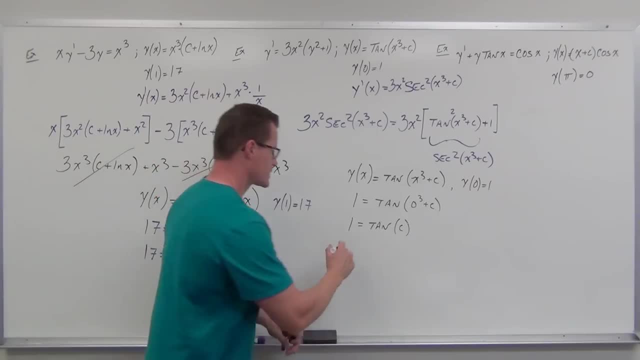 I'm thinking It's got to be pi over 4.. So c is pi over 4, because tangent of pi over 4 is 1.. Now we rewrite. So we're here, Remember, I rewrote it. I always rewrite. 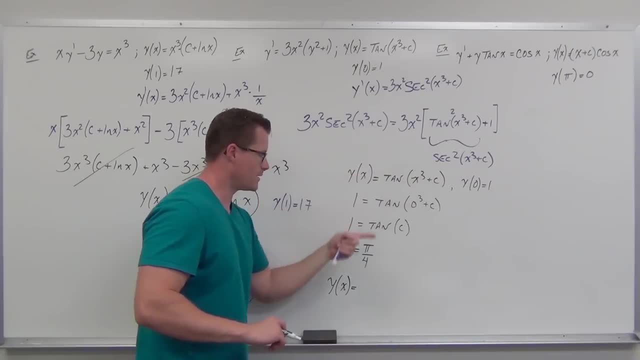 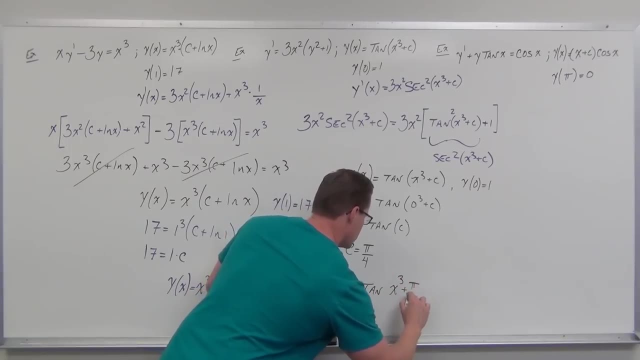 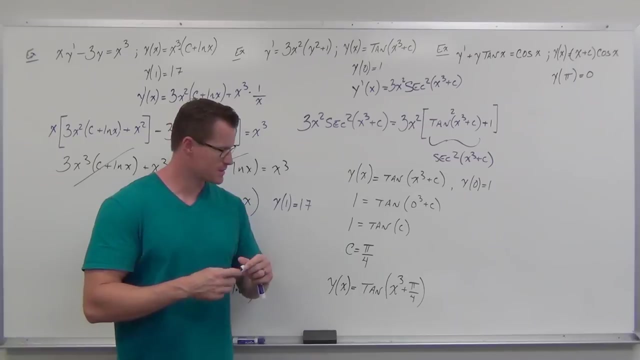 I verify, Then I solve for c. I always rewrite And then at the end I just replace the c. So that is a particular solution. Notice how solving for c gets rid of our arbitrary constant. We're good to go. That's what we're talking about. 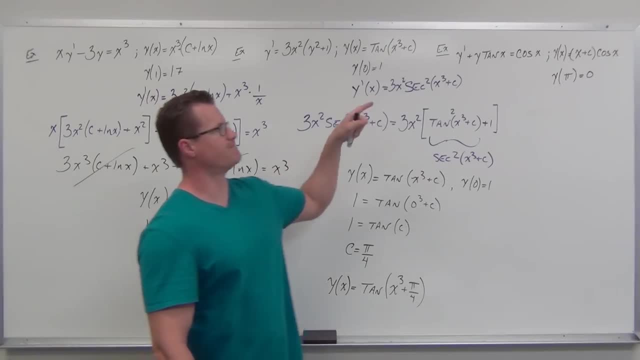 That's a particular solution. If you haven't, man, I'm really going to just beg you to try that one on your own. I'm going to erase it a little bit and give you some time to pause the video. Try it if you haven't already. 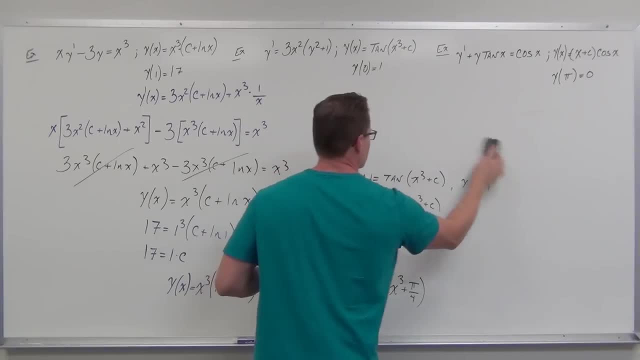 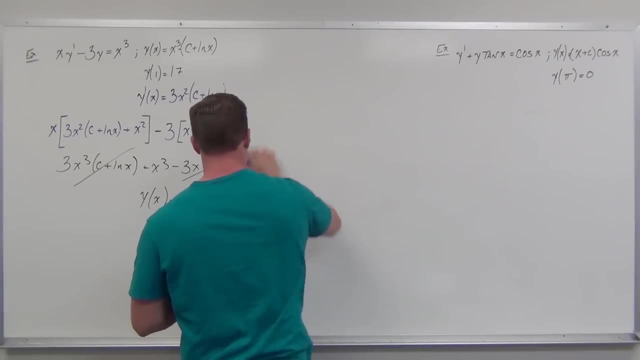 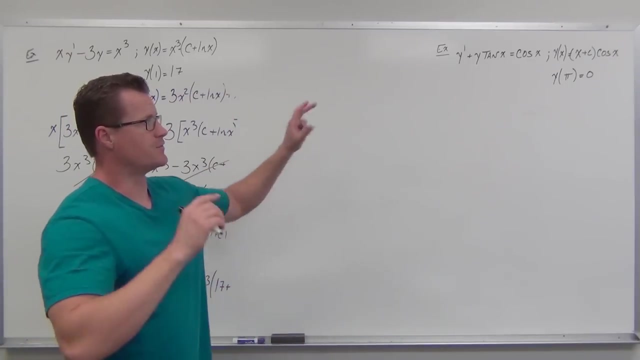 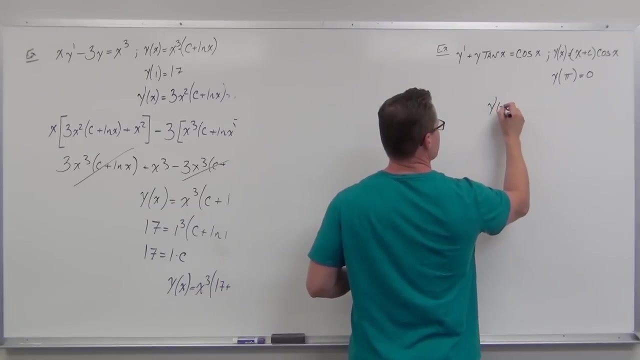 Here we go. So here we are. Let's take our derivative, Let's plug it in, Let's verify. first Let's solve for c, second Let's rewrite it last. Again, we have that product rule going on. There's a function of f. 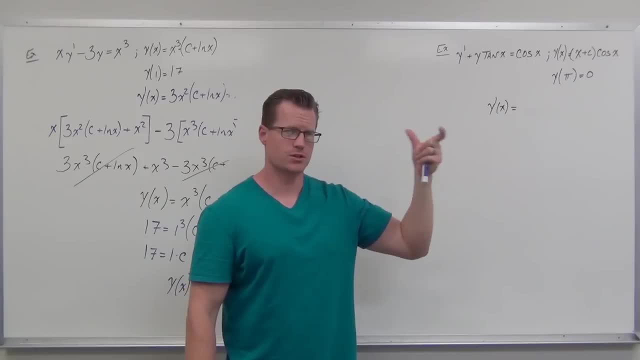 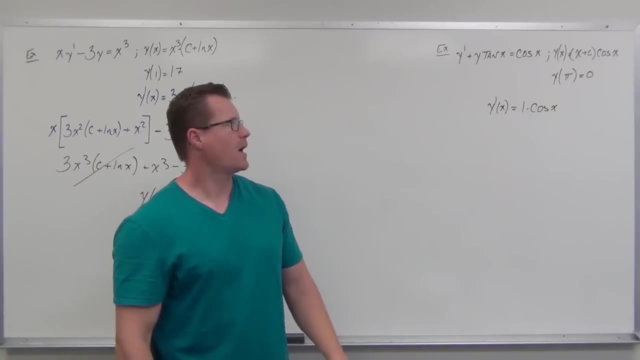 There's a function of x times another function of x. The derivative of the first, the derivative of x plus c, is 1.. 1 times cosine x. And then we're going to take the first function, x plus c times the derivative of the second. 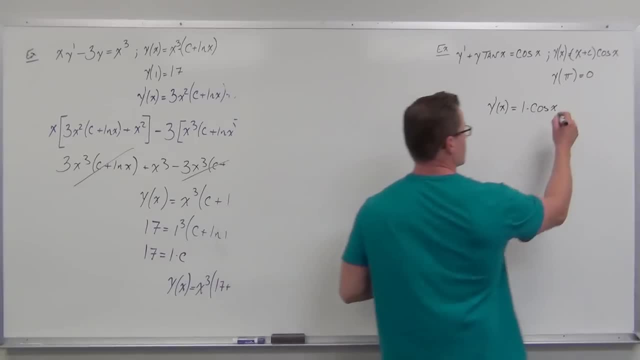 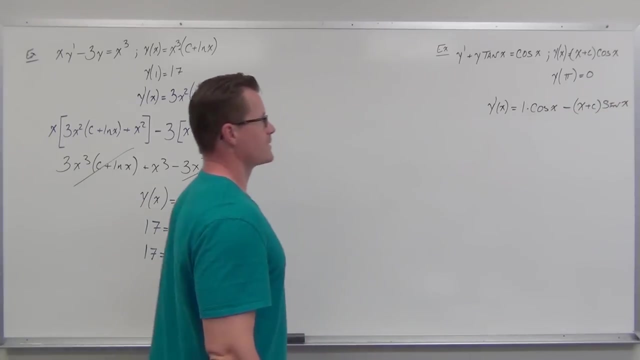 Well, the derivative of cosine x is negative sine x. So I'm going to put minus derivative of the first times the second plus the first times the derivative. So I'm going to put minus derivative of the second, which gives us that minus there. 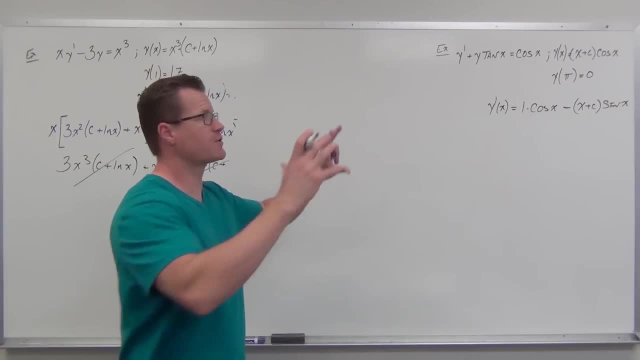 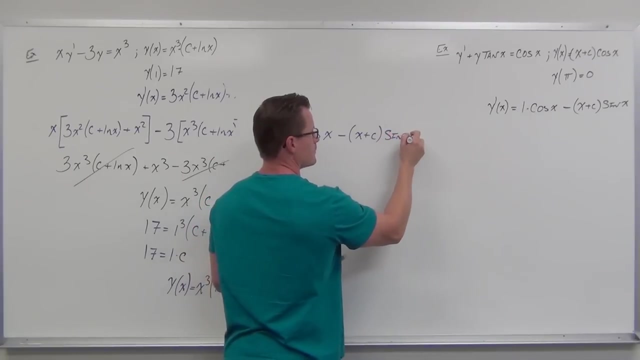 So that's our first derivative. Thankfully we don't have to take the second derivative, We just have to plug that in. So if we do that, it says take the first derivative. That's all of the stuff we just did Plus. okay, so this is our first derivative. 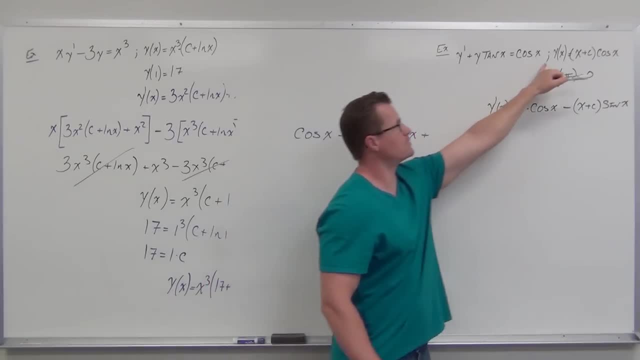 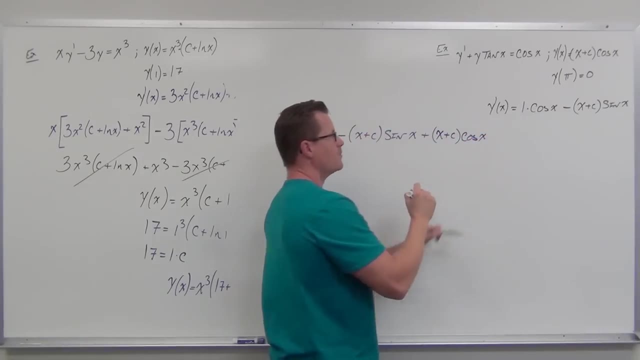 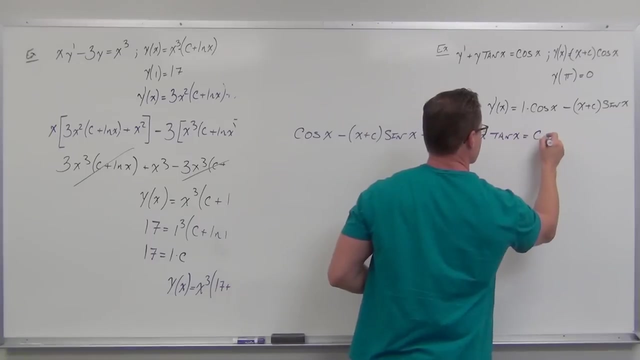 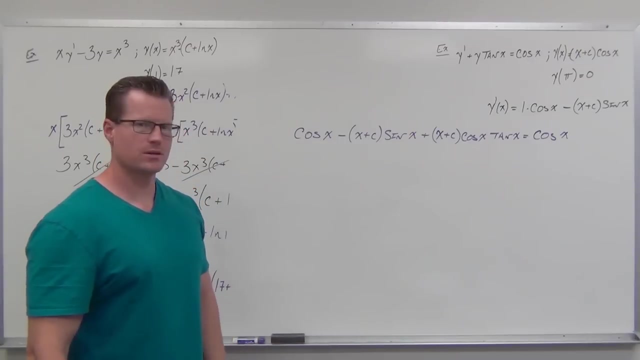 We're done with that. Plus Multiply, That's your original Multiply by tangent x, And that should yield cosine x. And again, this doesn't look quite right. Well, nothing cancels, Leonard. What in the world are you doing to me here? 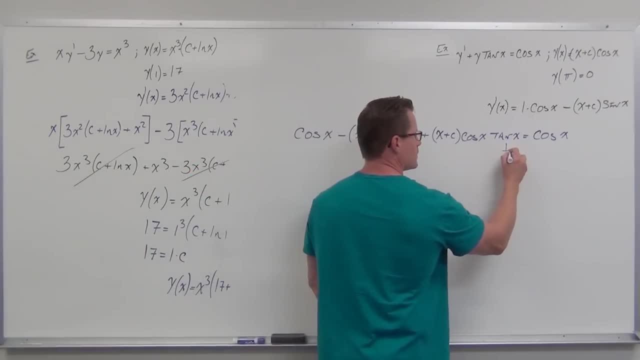 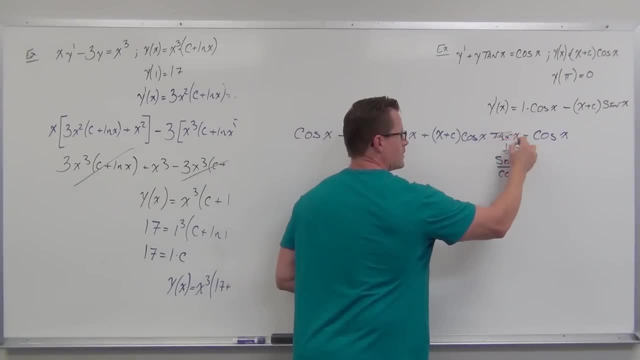 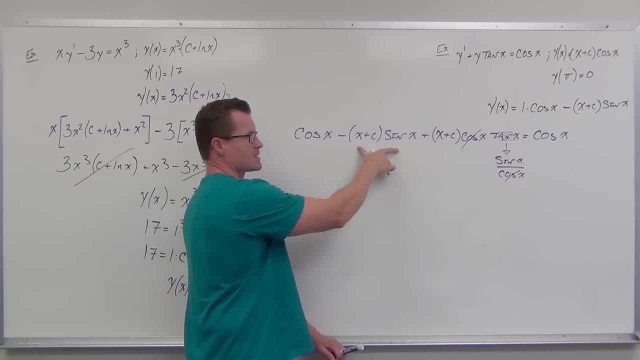 Well, the cosines are gone. We're going to get cosine x minus x, c x plus c sine x plus x plus c sine x. Those cosines are gone because that's part of tangent. Those cosines are gone because that's part of tangent. 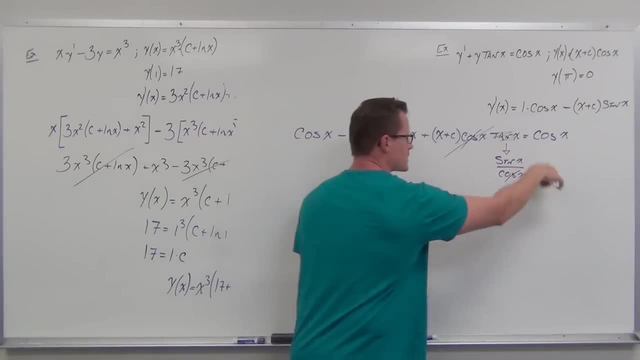 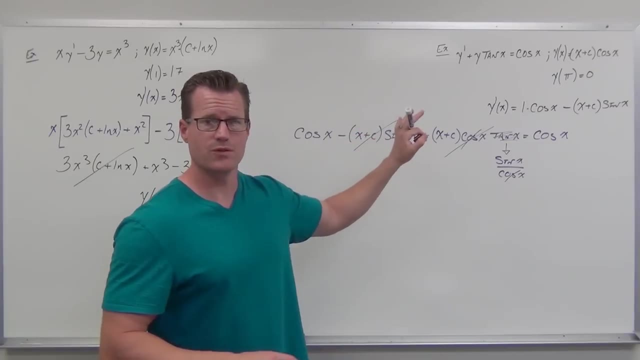 So we get rid of those. We get cosine equals cosine And that's all you have to do. That's verifying. This is not fancy-dancy, Just making sure that we got everything. that when you plug in the derivative in the original function. 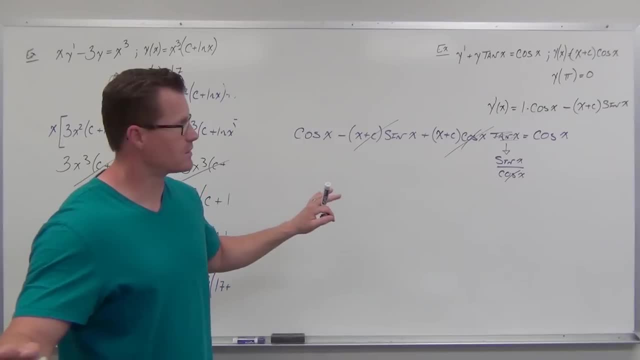 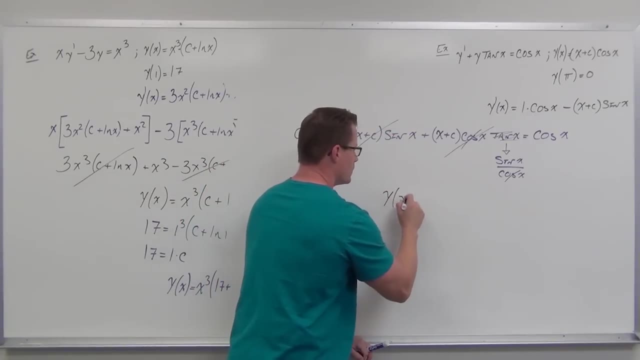 that you actually have a solution there. It's a waste of time to do anything else if you haven't checked that. Now that we've done that, we're done with that differential equation, We have our solution. We know that. that's it. 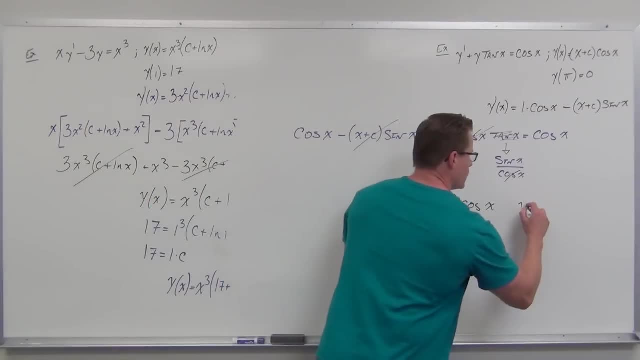 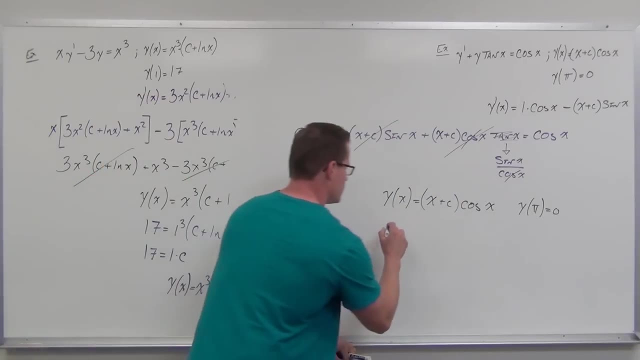 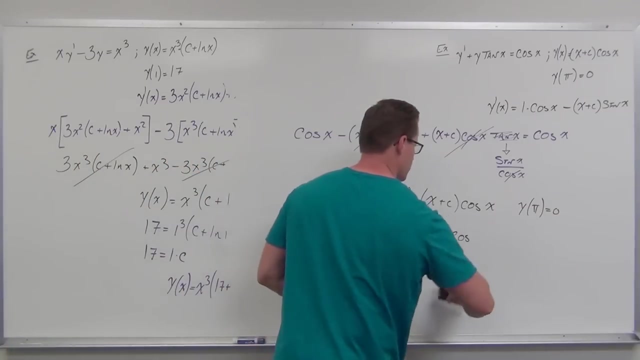 That's our general solution. We just need to find c. We can always do that with our initial condition. We know that when x is pi, that y is 0.. When x is pi, I guess I should replace all the x's in the puzzle. 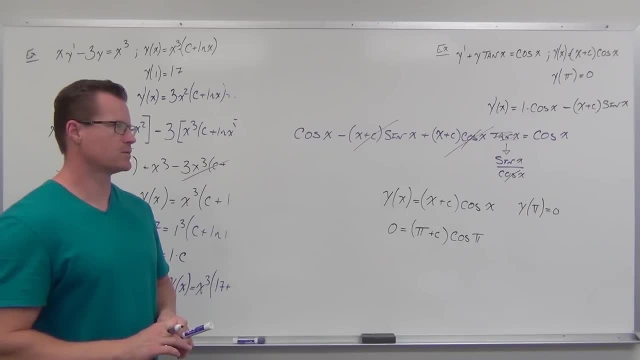 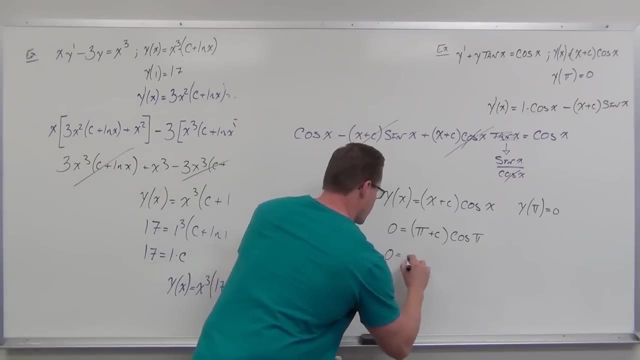 Do you remember what cosine of pi is? So sine of pi is 0, cosine of 0 is 1, cosine of pi is negative 1.. So sine of pi is 1, cosine of pi is negative 1.. So c is negative pi. 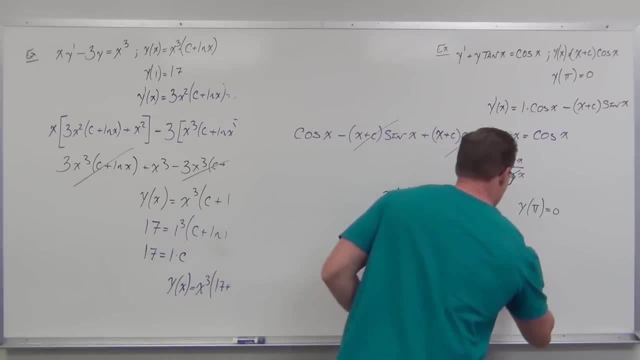 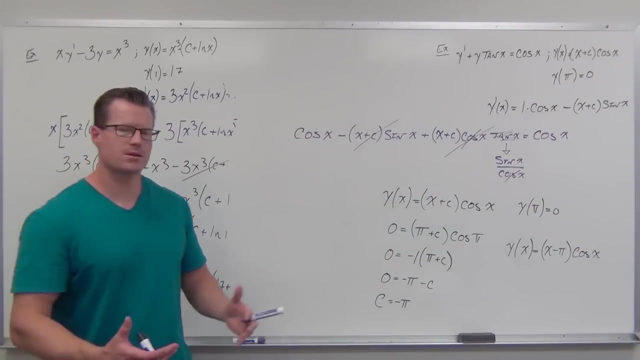 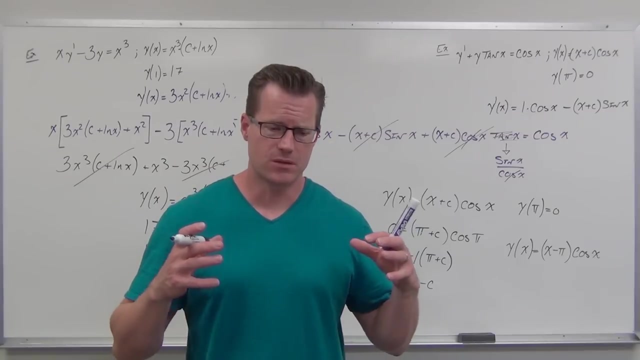 We can rewrite our general solution. So we can rewrite our general solution. with our c, We get a particular solution to our difference of equation. I hope this is making sense. That's about as much as I want to show you on how to find particular solutions given. 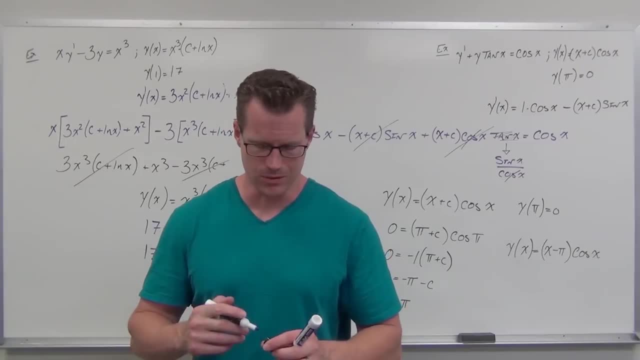 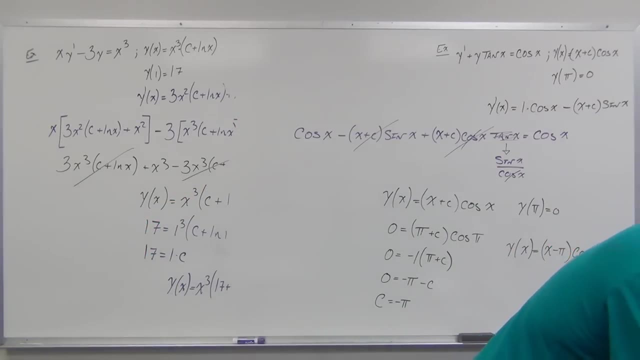 some initial conditions, some initial value problems is what they typically call those. There's one more. It's kind of a weird one, sort of for fun. Sometimes you'll be asked to do something like find all the values of a certain variable that make this a solution, and we're. 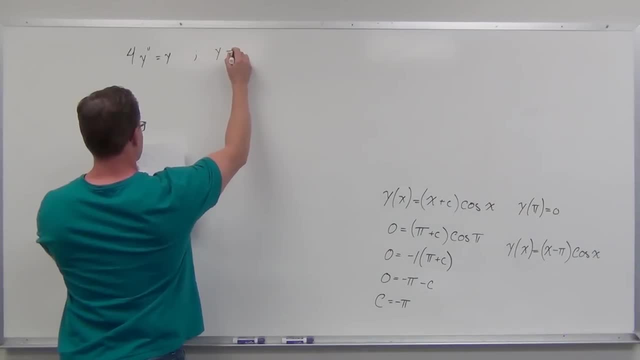 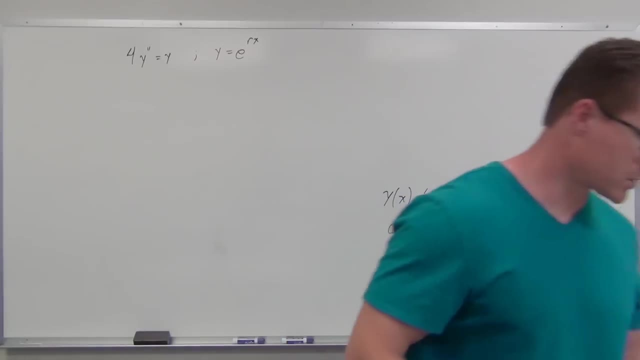 going to try one of those right now. I think the only reason why I'm doing this is because sometimes you get weird stuff. You're not used to it. You just don't know where to start. Not that it's really hard, It's just you don't know where to start. So how in the world do we find 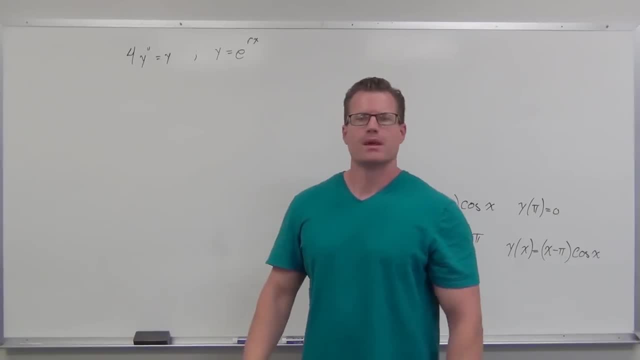 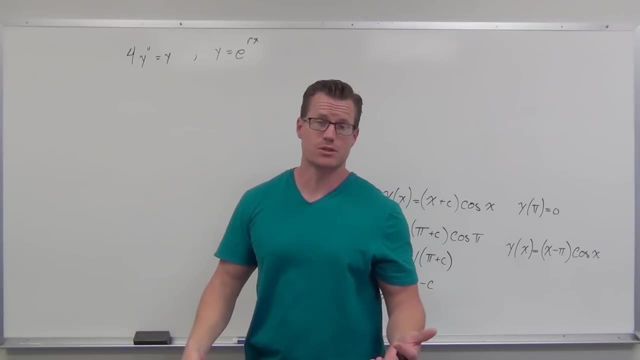 all the values of r that make this a solution of that. Well, just follow the process that we just did, okay, Find the second derivative, plug the stuff in and then you will eventually be able to solve for r. I'm going to show you one of them. The rest of them are very similar, if you have. 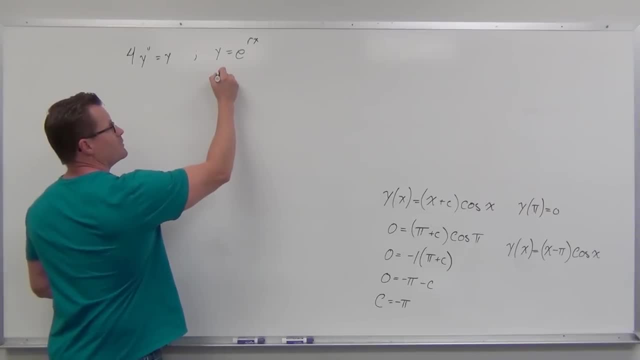 questions to ask of you like this. Let's find the second derivative. The first derivative, remember the chain rule. The second derivative gives us r-squared. So, first derivative, we get the e to the r-x back, but the derivative of r-x is r. Do that again.